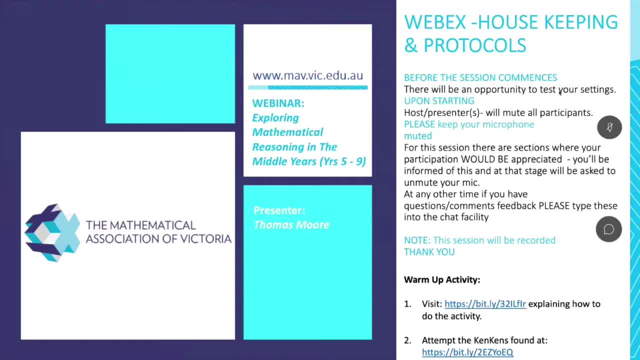 and he owns his own maths education company called Engage Me Mathematics. On top of all that, Tom's also in the process of completing his PhD. He truly loves what he does and he was born to do what he does, And that passion always comes through when he presents. 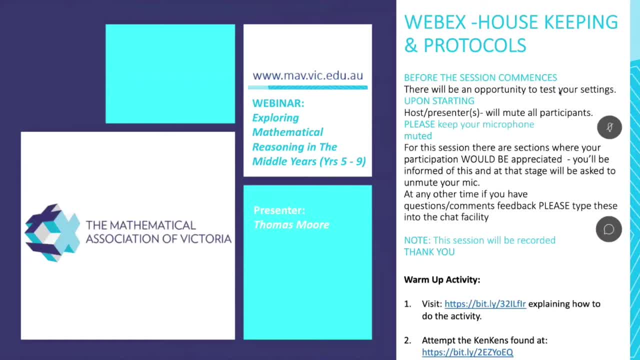 I was really lucky to work so closely with Tom on so many different projects and I've been really lucky to be involved in those with Tom as well recently. Just a few housekeeping things before I pass it over to our presenter. I have muted you all on entry. I can see some. 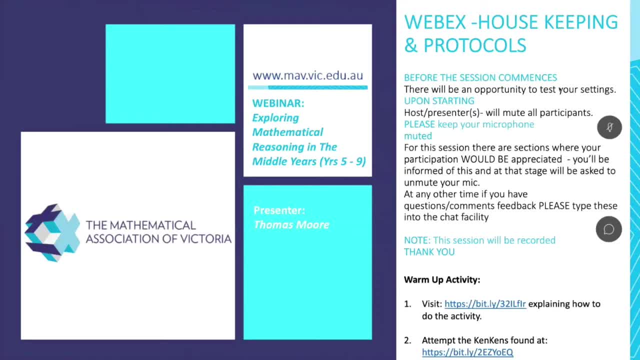 of you are unmuting yourselves already Just going to mute you. There we go. Just please keep your mic muted throughout the webinar. Hi, my name is Daniella. I'm a second year Mathematics Education Consultant at MAV. I'm here with Tom Lowin and one of my partners. Can you give a quick introduction by name? 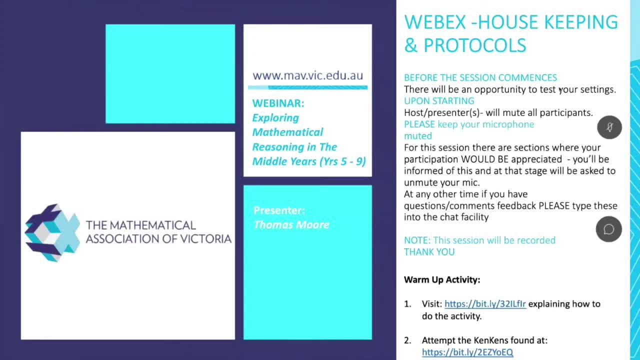 See what's out there. There is an introduction there in the presentation. There will be opportunities- I'm sure, Tom, you'll let me know it soon as well- for them to unmute and contribute at certain times. Is that right? Yes, that is correct, and I'll let you know sort of one by one, because we can't. 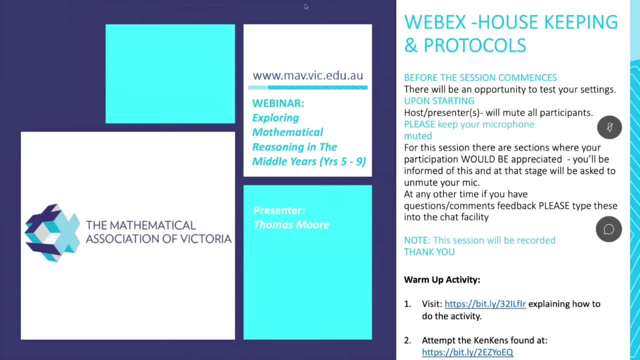 be having 144 people doing that. We've got quite a large number of people registered for tonight, so we're expecting a lot of you. So maybe you won't all get that chance to have a say. there will be opportunities, and if there isn't opportunities to speak verbally, you can always. 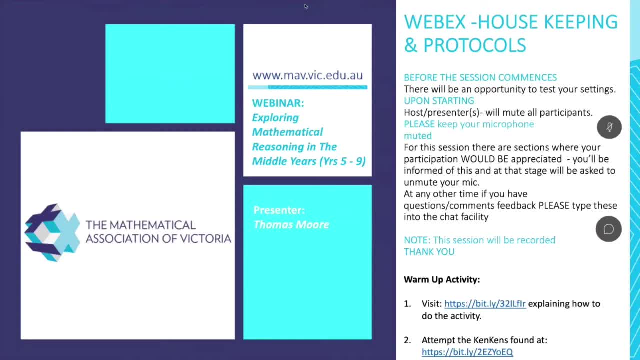 use the chat box and we'll try to get to every one of you through that. um also, this webinar is being recorded and you will receive the recording as well as any resources, including the slides that we will use today, so there's no need to frantically write anything down. you will receive. 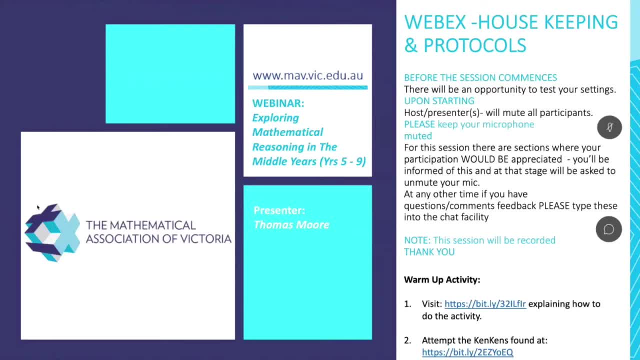 all the resources. okay, over to you, tom. good luck, okay, excellent. thank you very much, daniella, for that amazing intro and if you wouldn't mind, could you just quickly type in the in the chat for people, if they can't hear us, to try logging in and then back out again. hopefully we can sort of get. 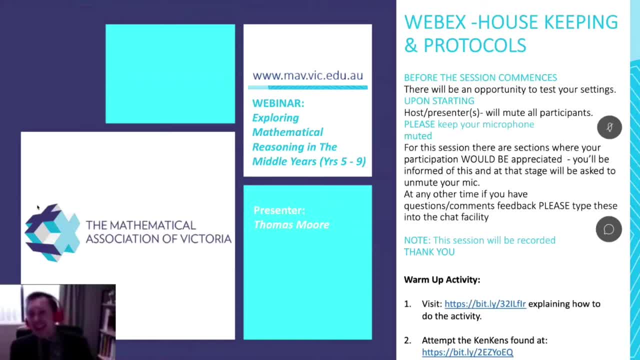 on top of those audio issue issues for people. but thank you firstly for those amazing things that you said. as i, as you went through and did, i thought, wow, geez, i've got to live up to this now. so there is a bit of pressure and i appreciate that. um, because you know, pressure makes diamonds. 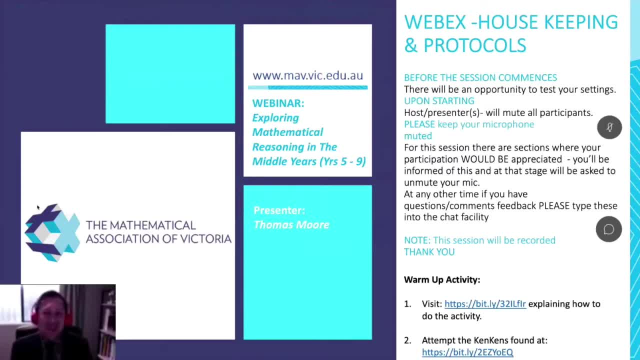 so hopefully, that's what we'll go for today. now, in terms of this, i'd also like to say thanks as well to everyone. i know that you guys are flat chat with your classes and remote learning and all of those things at the moment, so it's actually a real honor to be able to present to all of you today and to 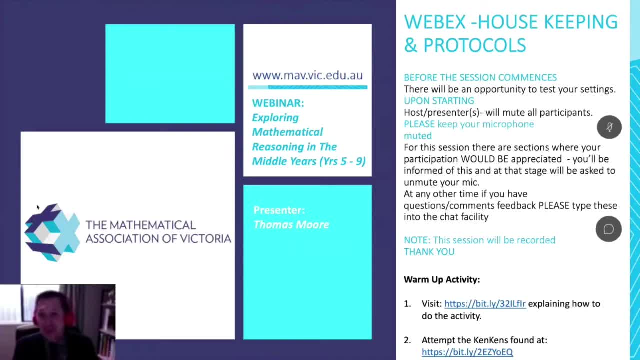 to know that you guys have been willing to give up all. you know the very little time that you have to be here today with us, uh, so hopefully you'll get something out of this. i've tried to make sure that i put it brought a whole lot of resources and stuff in so that you can take. 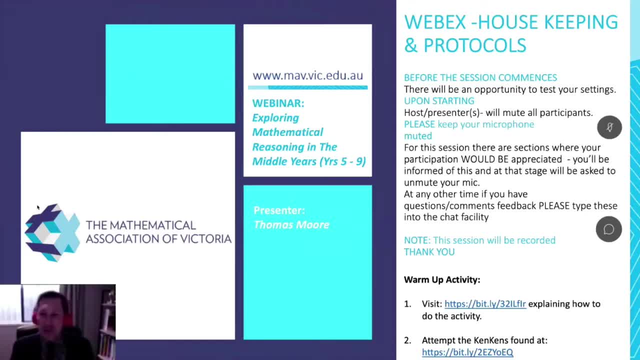 something away. so hopefully you guys went through and had a bit of a go at the warm up, warm up activity. if you didn't, though, it's not the be all and end all, it's just: you guys went through and had a bit of a go at the warm up activity. if you didn't, though, it's not. 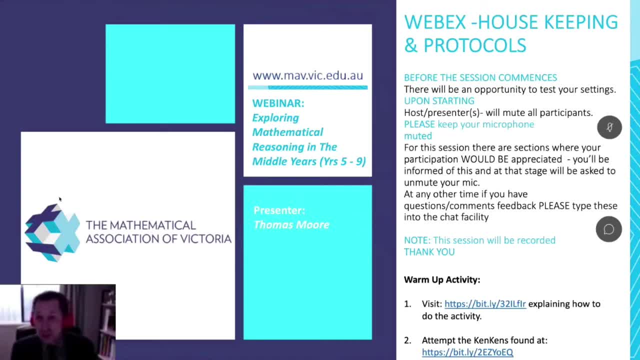 a great little reasoning activity that you can use with your students- and i've used that with students all the way up to year 11- and you know all it's involving is some simple addition, but there's some reasoning that goes into that, that makes it challenging and that makes it. 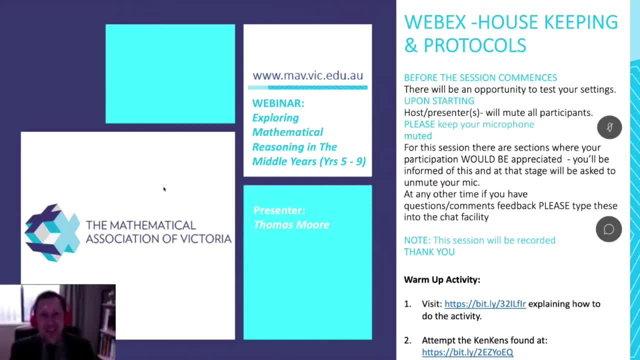 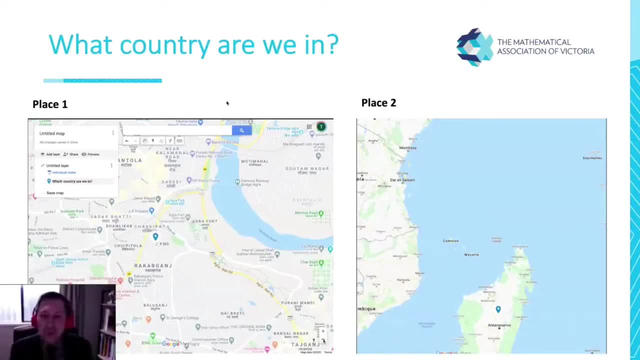 engaging. all right, let's get on with the presentation, so i'll just click on this. what i've got here on my screen are two images. now, these images are located somewhere in the world and i've zoomed right in on a certain place, and your challenge right now is to have a look at this and to try and figure out where in the world. 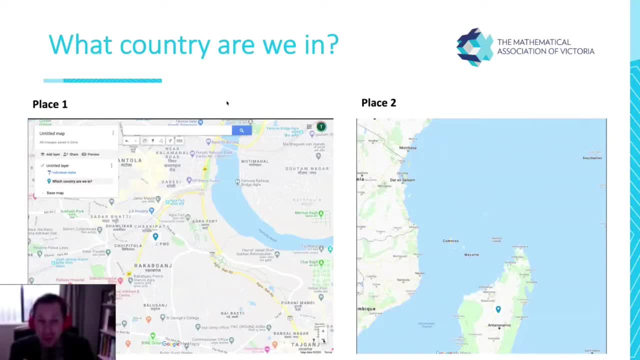 i am for these two places, but i'm going to give you- don't answer this before anyone- um don't. i'll give you about 10 seconds before you put it into the chat, but after 10 seconds i'll let you know when. type in where you think it is all right, have a look around, i'll give you 10 seconds. 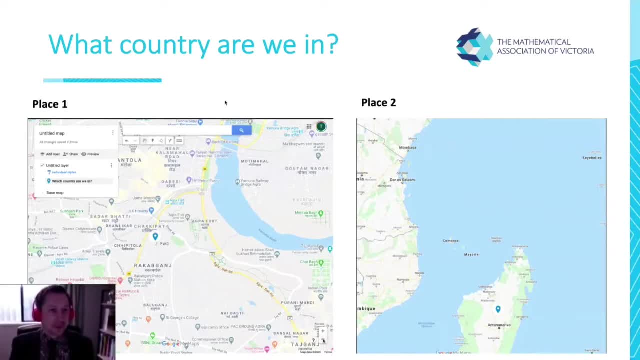 all right, a couple of people were pretty. you can now start entering in those answers. so if you think you know whereabouts we are, there we go. so i can see a number of people putting in egypt, africa, madagascar, india. so let's now have a look at where we are for each one of these places. i'll just go ahead and we'll 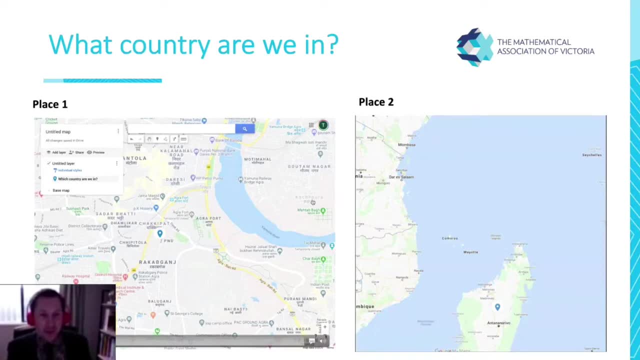 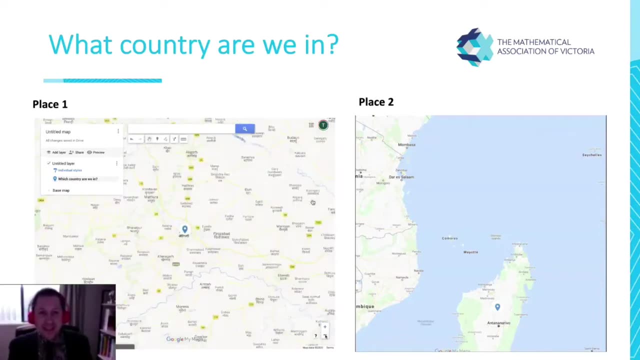 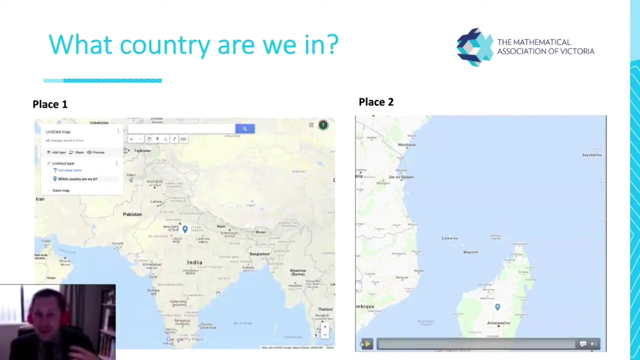 press play on this one. i'll zoom out and we'll have a look at where we are getting there and of course, we are in india, all right. so for the next one now, of course, with the india as well. there might have been a couple of hints in terms of you might. 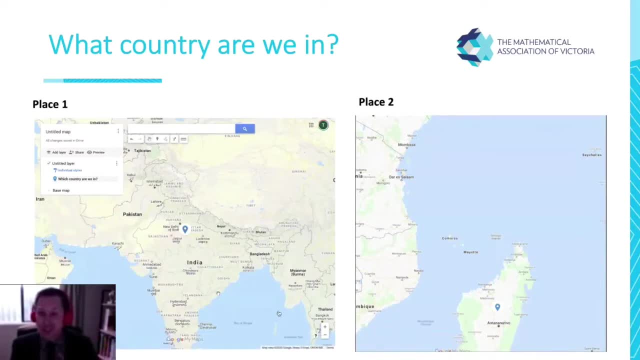 have seen taj written, or maybe you knew that agra was part of india, where the taj was. let me show you this one. this one was a nice, easy one. i wanted to give you a little bit of information in terms of seashells being around and mozambique being there. so of course, we were in madagascar. now i'm 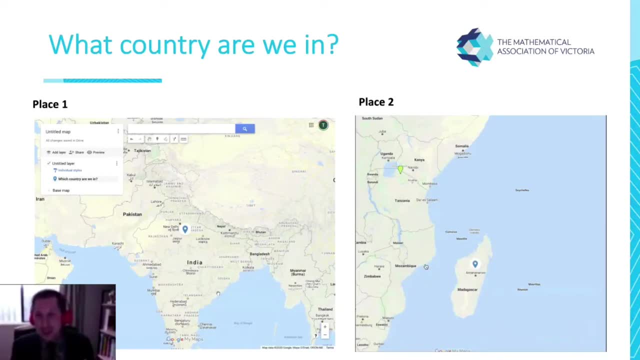 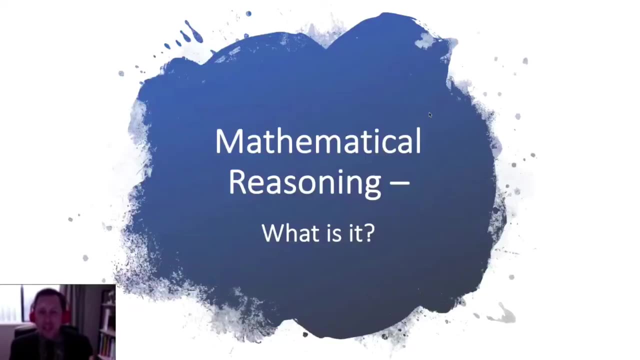 going to come back to this and how it relates to reasoning. in a second i'm going to come back to it, but before we do that i just want to get your thoughts on what mathematical reasoning is. so i've included all the proficiencies here from the victorian curriculum and- and i sort of highlighted 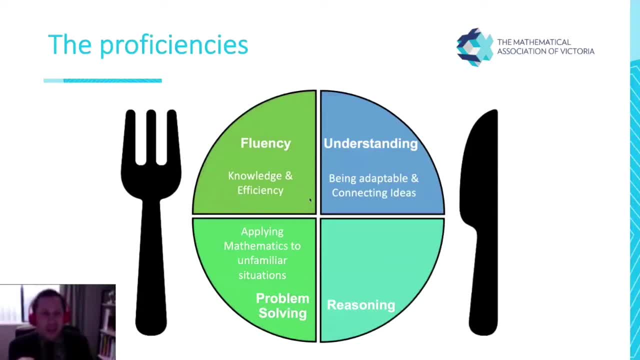 the main sort of things that i got from them when i was reading through the proficiencies. but i'm interested to know what reasoning means to you, so feel free to put into the chat what reasoning is to you. so i've got sushma saying language. 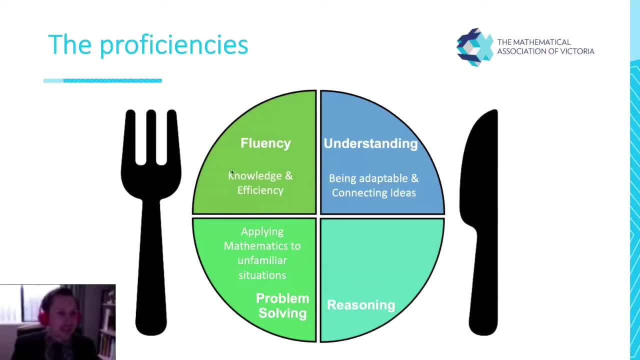 making sense of communicating your thinking, number sense. justifying something makes sense, being able to understand and express your thoughts, describing your thinking, logical thinking, explaining your thinking using facts, etc. proving your solutions. awesome, all of these things. you'll see what, when it comes to looking at the um, at the vcaa statement, you'll 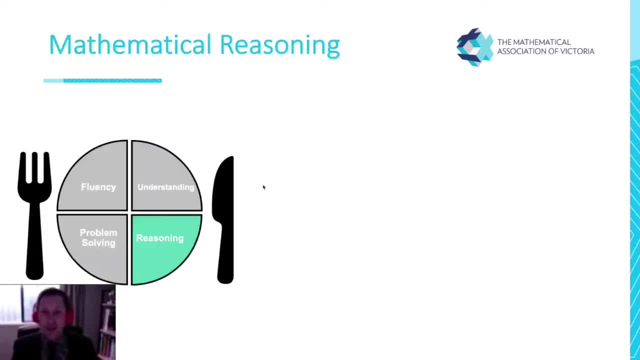 see all these things come through and in fact i'll bring that up for you now. i'll give you a moment to sort of explain what reasoning is to you. so i've got sushma saying: language making sense of communicating your thinking number, sense justifying your thinking number. 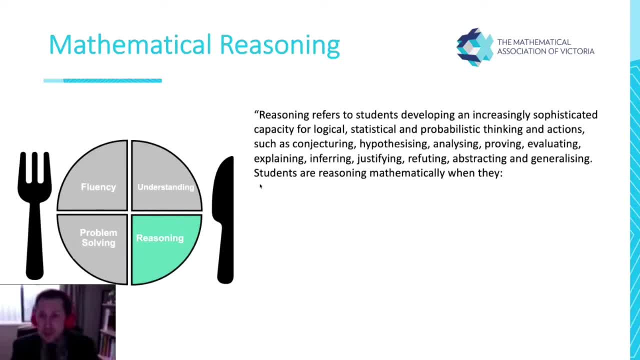 read that statement there. in fact, i'll read it out as you guys get a chance. so reasoning refers to students developing an increasingly sophisticated capacity for logical, statistical and probabilistic thinking and actions such as conjecturing, hypothesizing, analyzing, proving, evaluating, explaining, inferring, justifying, refuting, abstracting and generalizing jesus. a lot there. 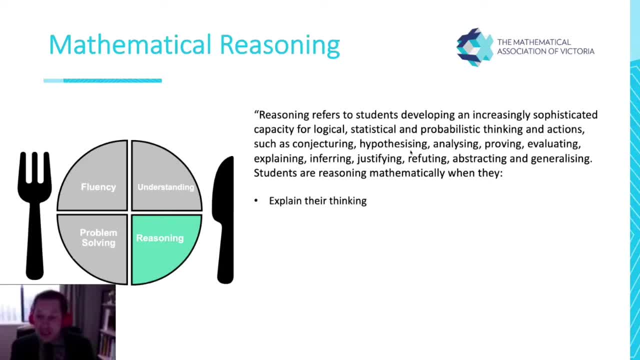 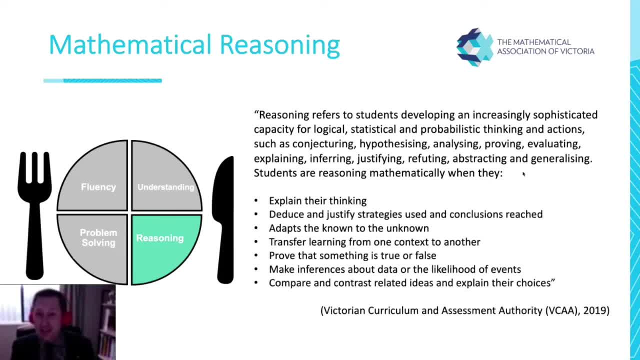 inferences about data or the likelihood of events and compares and contrasts related ideas and explain their choices. now i probably went through that very quick for you, but it is all on the vcaa website and you will have seen this no doubt before. but to me, reasoning is much like what we 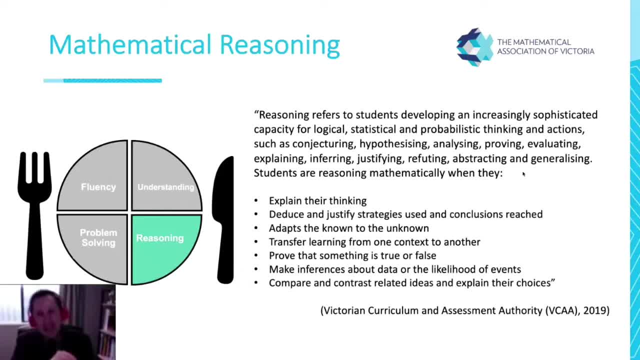 did in that first chapter of the vcaa statement. so i'm going to give you a little bit of an example of what we did in that first task, where we started off looking at the map and we're trying to make sense of information that's around us in order to be able to take a step back and see the bigger. 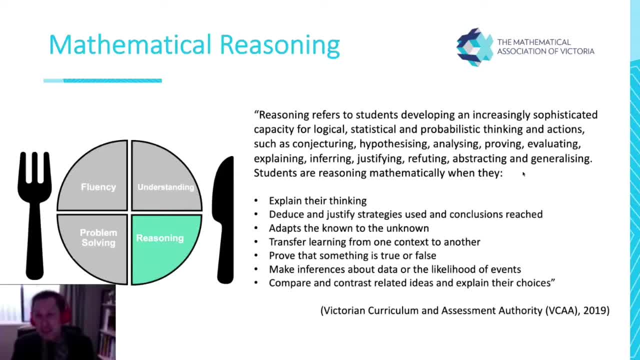 picture to make sense of the landscape that's around us, or in other words, i guess, to see the forest through the trees. reasoning is that process of being able to look at things, muddle our way through it and then be able to make sense of it in in its bigger picture. and, and we do that through 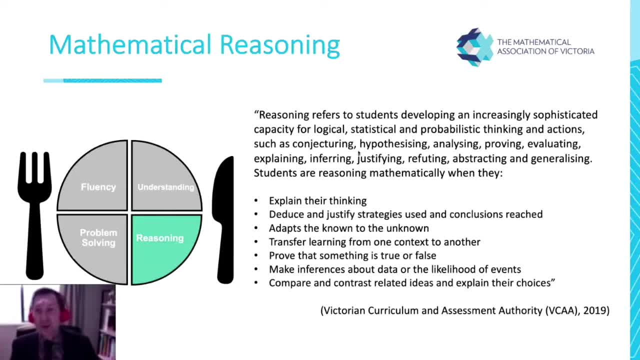 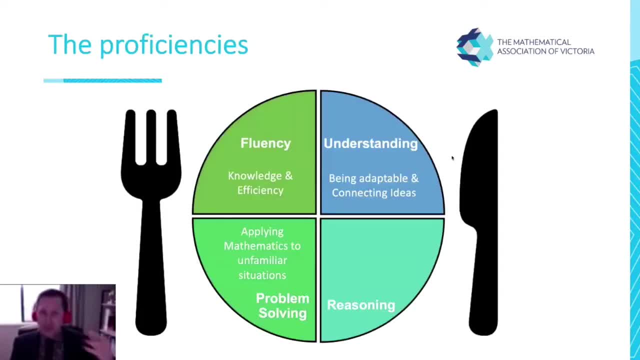 all of that and we do that through all of that, and we do that through all of that, and we do that through all of these different words or verbs. i guess you could say that we can see up on the screen here now you've noticed. and so, in terms of what i did when i went through and looked at the vcaa thing, 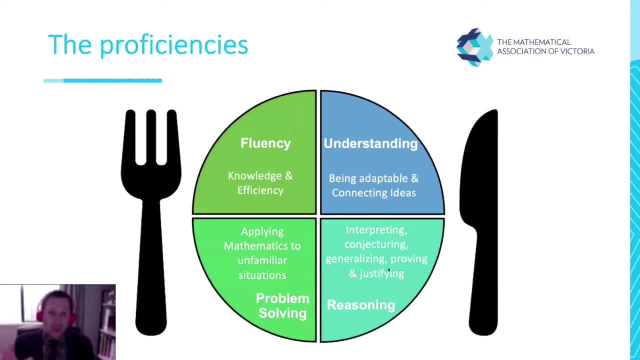 um website. i just sort of put it down as these things. now there's more to it, but i just wanted to put it all on one nice plate and you'll see that i've got the knife and the fork. and the reason why i do this is because i look at the proficiencies on the vcaa website as being sort of 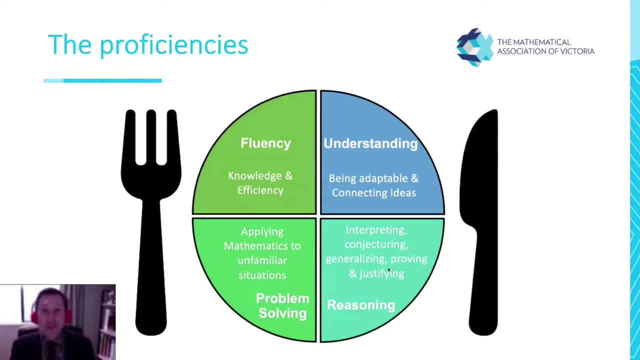 like the healthy, balanced nutrition, and i'm going to show you a little bit of that in just a moment. um, i'm going to show you a little bit of that in just a moment, so let me just give you a few quick examples of what we would give to students to help them. 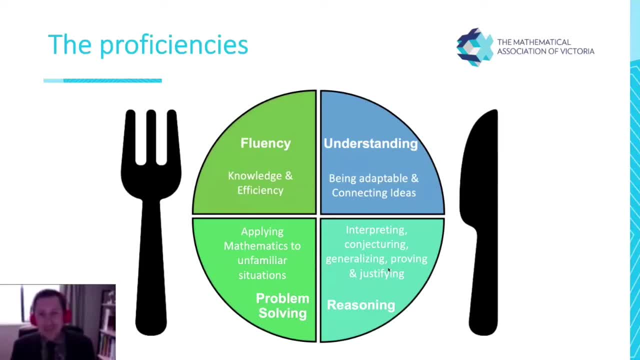 understand mathematics, and so the first thing we would give students is a little nutritionist meal that we would give students in terms of mathematics learning, for example. if all we give them is fluency, they'll miss out on all the other stuff that is so important to knowing and understanding. 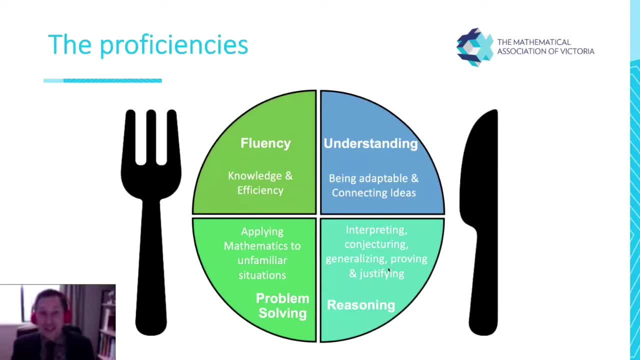 mathematics and i'll tell you a little story as well. when i first started down this journey, i actually gave a lot of students. i've spent a lot of time on the reasoning side of things and in fact i i neglected the understanding, fluency and problem solving. now i love reasoning. i think that's one of the most meaty parts of the vcaa. 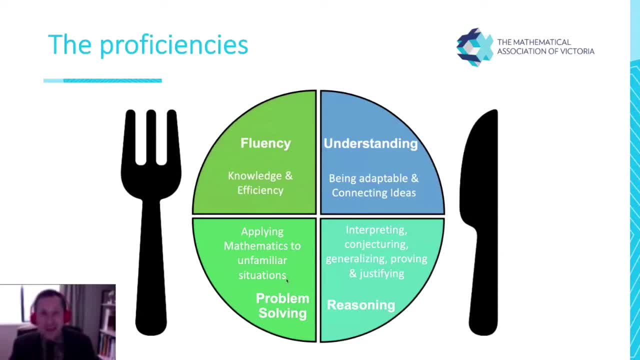 meal. all right. reasoning to me is kind of like the hero on the plate. it's like the you're not as lasagna or your, your mum's uh, sunday roast that you know it is the best. okay, oh okay. i can see that i'm cutting in and out. can people? is that common for everyone? can i just get it in the? 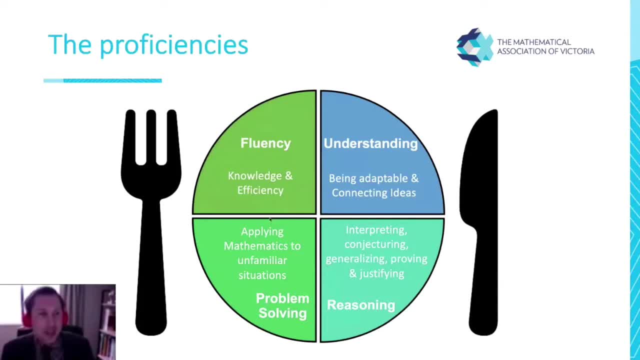 comments. if i am cutting in and out, okay here, all right. so it might be some people thank you for that. if you, if i am cutting in that you might need to just change your audio settings. but reasoning is part of the meal. now we can't just focus on reasoning like we just can't focus on fluency. we 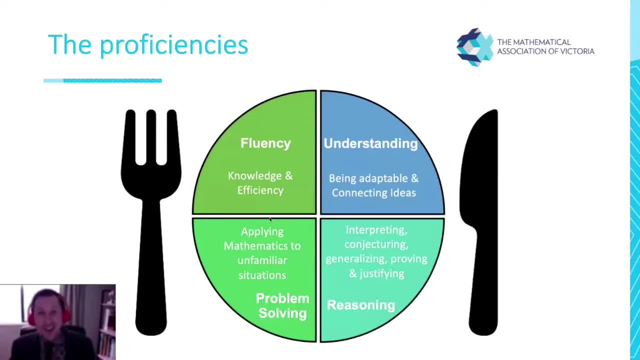 have to have a nice balanced nutritionist diet, nutritional diet for our students. and when i did this, when i focus on reasoning, just reasoning- what happened was students pushed back because they needed that balance of all the other proficiencies. so it is important to make sure that we're constantly looking at what we're teaching and thinking about well which proficiencies 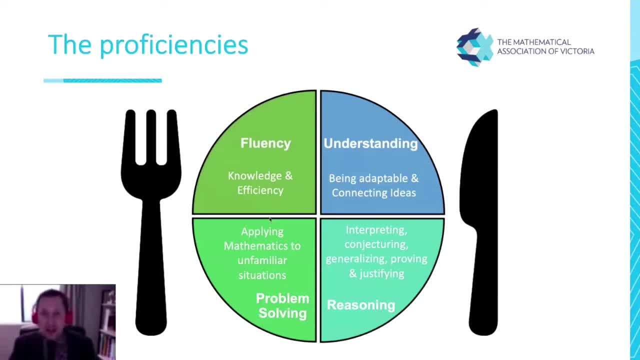 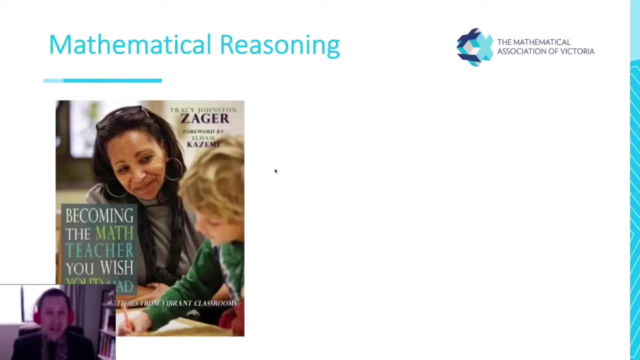 am i mainly addressing and making sure we deliver a nice, balanced curriculum in terms of working mathematically, okay, so in terms of um, in terms of reasoning as well. i've read this book recently. it's by tracy zagar. it's becoming the math teacher. 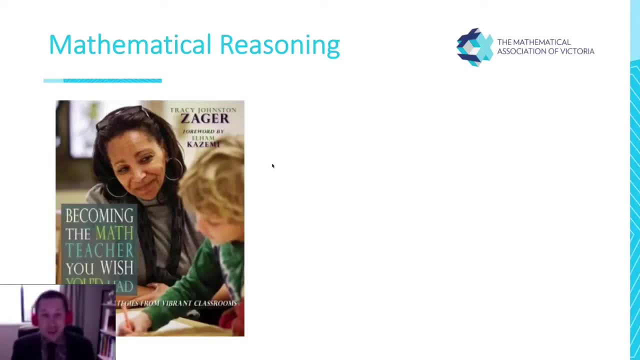 you wish you had, and i really enjoyed this and highly recommend it to anyone else who's interested in reading something along these lines. it she described um reasoning as being similar to writing for students. so when you go through and you and you write, like i know, i write emails and quite often i'll write the first little bit and then the next little bit. 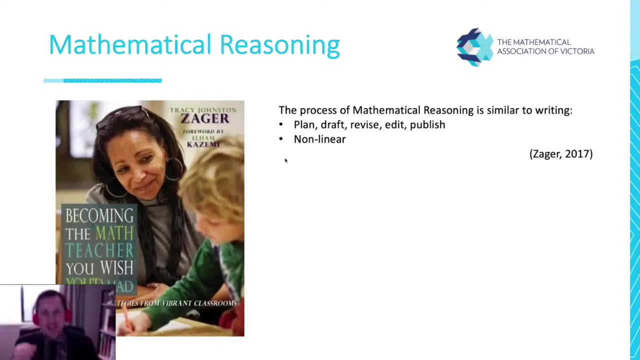 but then i'll try and change it around, so it's not quite a linear thing. in fact it can be circular, it can come at it from different angles. so reasoning is about coming at things from different approaches and it's not always linear. but what i find is, when i work with students and when i work 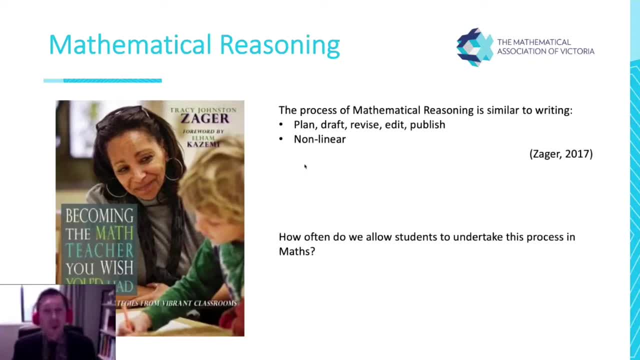 with schools that this process doesn't happen all that often in in the classes, and that's actually been backed up by some of the research that di seaman's done as well, and she said that activities involving mathematical reasoning are really given the attention that they deserve. so this is why i'm 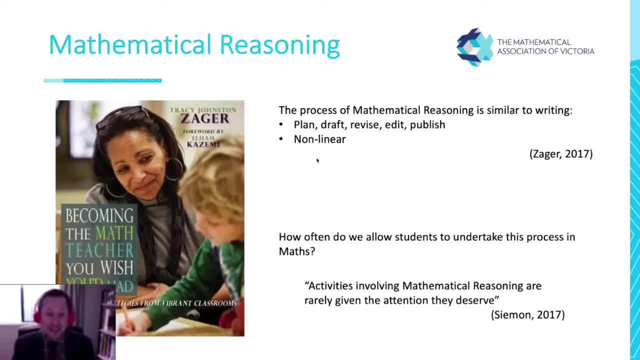 focusing- or i chose to focus on- reasoning tonight, because i really think that this is an important area for us to work on as a profession. now, that's not to say that doesn't happen in every classroom, or that happens in every classroom, obviously, and the people that are here are here because they. 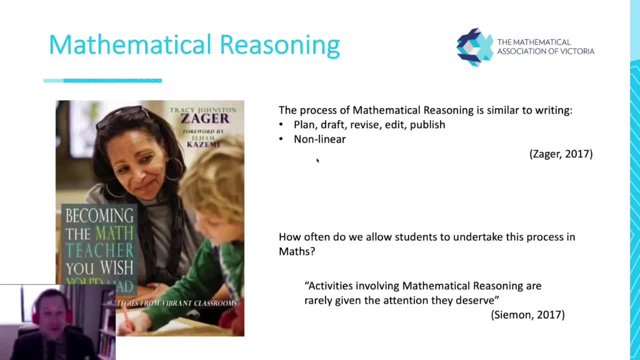 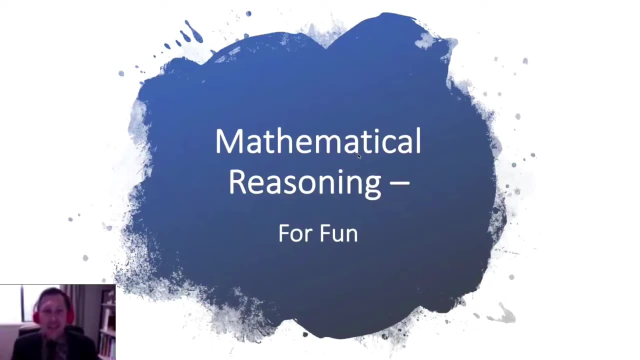 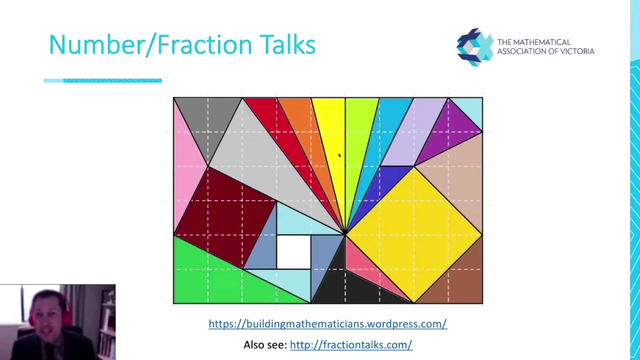 want to learn more and they um, and they obviously value reasoning as well. so it's not to say it happens in every classroom, but it's an important thing to keep in the back of our minds. so you can see, here is equal to one. that's one square unit. my challenge for you is to just once again: 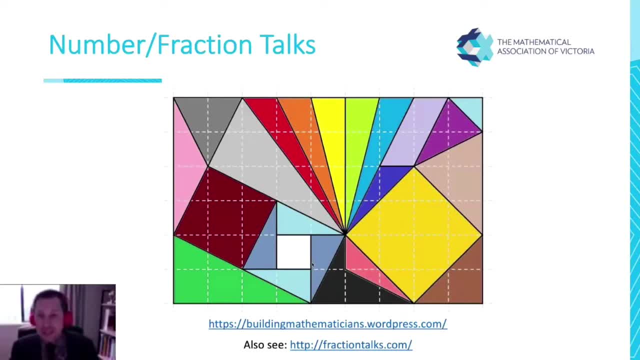 don't write it straight away. give yourself about 10, 15 seconds to have a look at it and i'll tell you when that time's up. have a look at it and try and put down what are the colors you think you could figure out if we know that this white square is equal to one. so i'll give you 15 seconds to go. 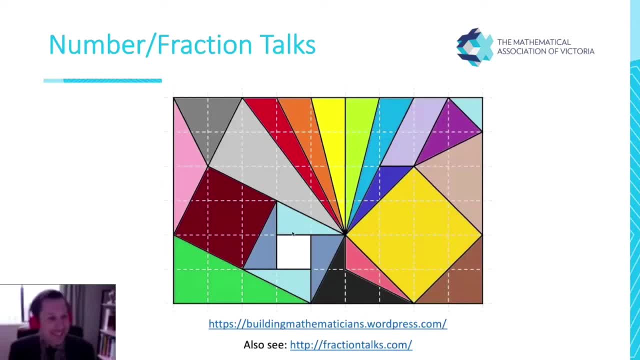 through and have a look. ah, awesome, erin's just used that one today. brilliant, so don't start writing anything in just yet, though. give you 15 seconds to have a look. let's down down to 10.. jesse, will there be hyperlinks to the resources you've referenced? by any chance? so i'm sure you've. 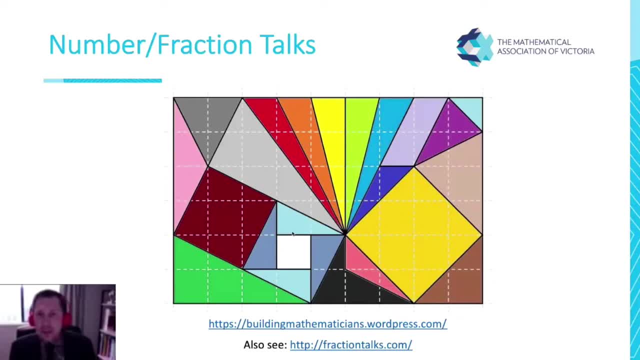 got a. do you have a resources or reference list at the end? yes, that, absolutely. there's a reference list at the end and you'll get access to these slides so you'll be able to go through all those um hyperlinks as well. excellent, now feel free to type in what. what can we see? what do we notice in terms of colors? 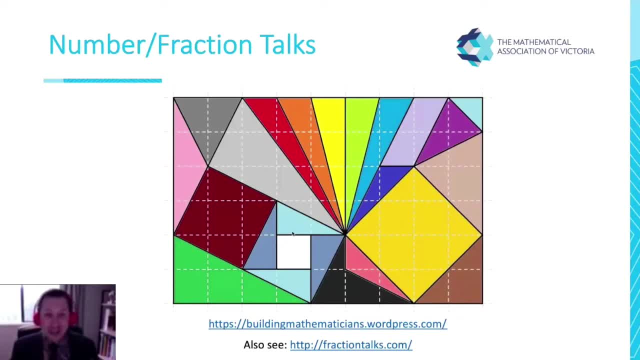 does anyone got any any thoughts in terms of what they think different colors might be worth? if we know the square is one, cool, so the brown is two. so that is this brown. here i can see one, and then this one here if we move this part over here. 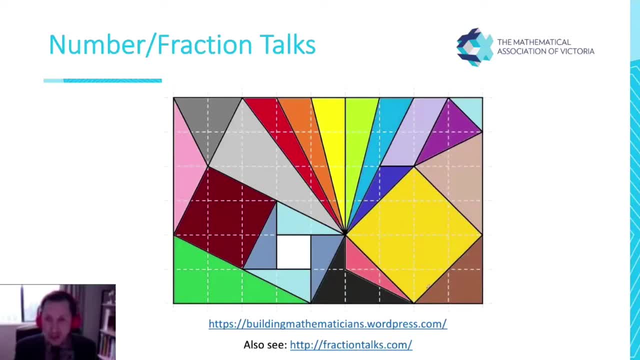 that would be two. in fact. i'm gonna bring the pen, so if i got this brown part here and i moved it over there, i could see two. top right grey is two. so the top right grey, uh, where? or would that be the left one? maybe i can see here. so if i put this one down there, 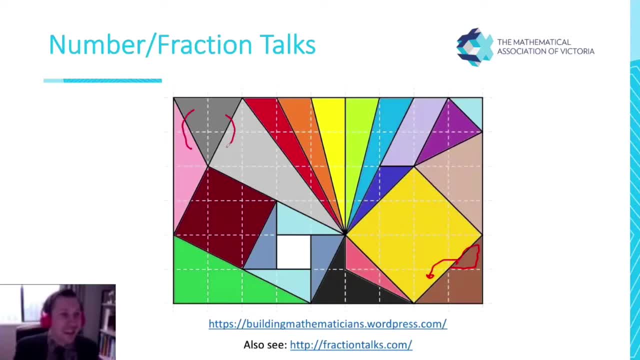 and this part down here i could see two awesome. blue equals two. oh, that's an interesting one. um, who put down the blue was two? someone able to? whoever put down the blue was two. are you able to jump on the mic and share your thinking? all right, just while we wait for that. so i can see a whole lot of things now what i'm. 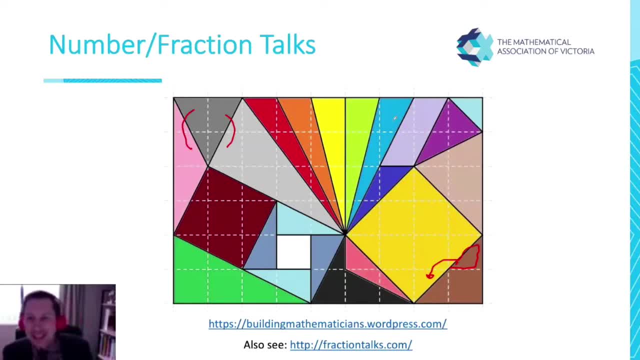 interested in is: sorry, tom. no, that's right, sorry, what was that? um, because i put down that the light blue in the top right is worth a half. okay, excellent, so you're talking about this one here? yep, and i think what they mean by the other blues it means when you look. 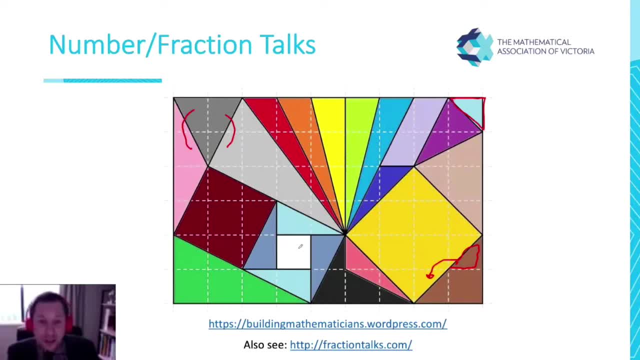 at the white square, the white square. so this one, yes, yep, hang on. so when you look at the white square and you look at the light blue on top and the light blue down the bottom, they're each worth one. so together that would be two and the blue. so you're saying i are 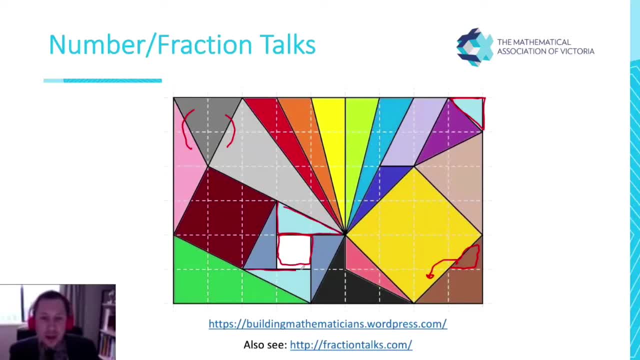 also each worth one, so together they would be two. ah, so you're saying, if i put this one here, down here, that therefore would be equal to two. and what was your other thing that you just said? sorry, the two blues on either side are the same, okay. 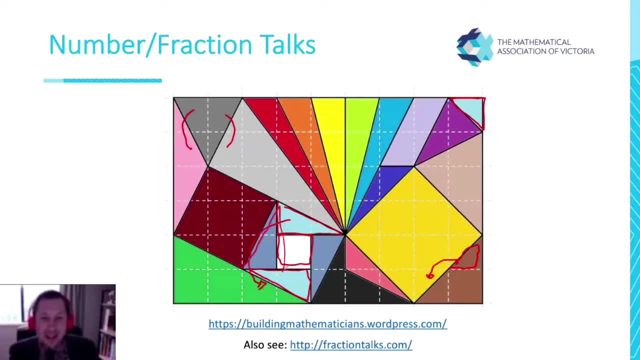 ah, okay, awesome. so you can see here that that and that would also equal to yeah, nice. so, and we know, of course, if, if that part, if they all these blues, so if that's two and that's two, that'll be four, and then we've got the white, here would be five. so therefore we can. 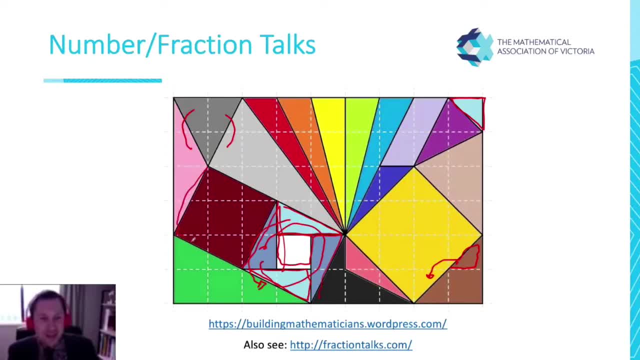 figure out that that's the same as the brown, isn't it? yep, nice, okay, very nice, all can solve. all right, are we allowed to use formulas for areas as well? well, absolutely, if you, if you know stuff, then you certainly can use the formulas, but at the same time, you can use the formulas for areas as well. 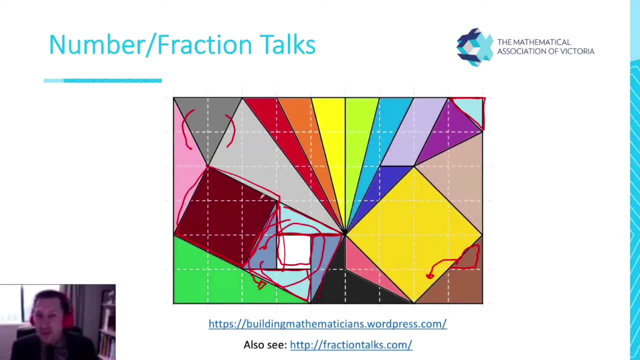 same time, it's good to use the reasoning in terms of: well, how else might we know? for example, how might i know that the yellow here? or how might i be able to figure out the yellow? or how might i be? if i know that, how could i figure out the orange? so it's a great way to 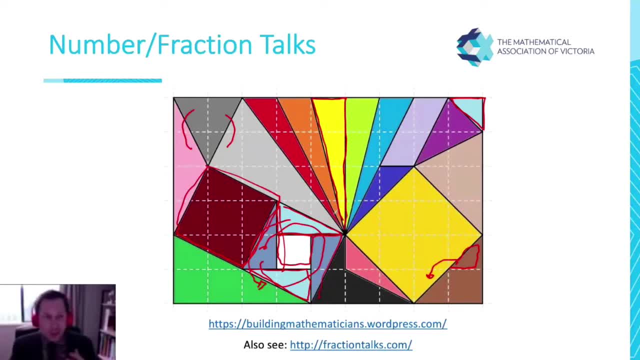 not only be able to explain it in terms of you, with formulas, but also if you can explain it in another way. my favorite one is this: this orange- sorry, the purple one here. does anyone want to have a go at the purple one? but colours are all two, okay, simon. simon, would you mind sharing your thinking for the purple one if? 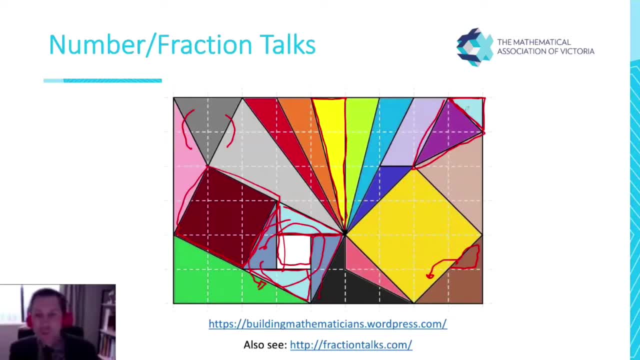 you could just jump on the mic or m heating or heading, if that's how you say it. sorry so yep, I can see that I haven't got a pen, so the one on the bottom left if you rotate the one above it down to fill in its hole. 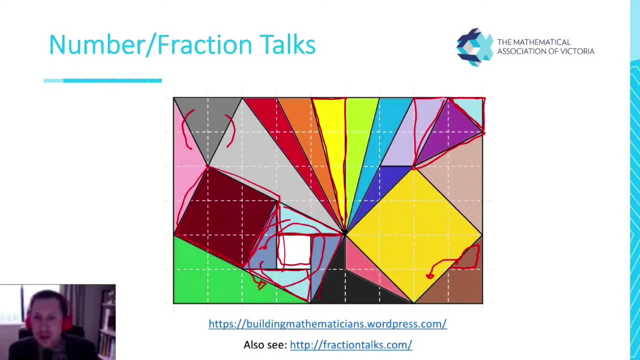 on the top left corner of it and then take the one that's second on the right down and spiffle it down. you've got a full one there, and then you add in half of the top right cube. Okay, so am I right in sort of saying you're using? 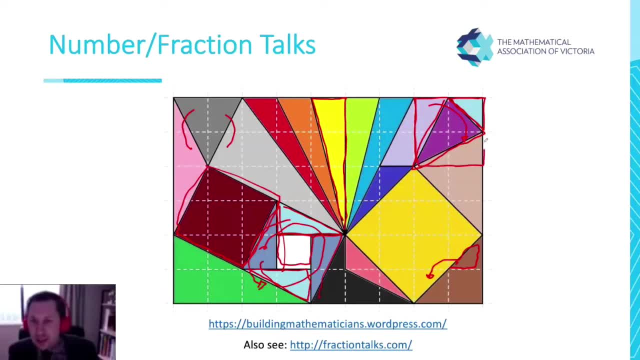 these four squares here. Yep, To be able to figure it out. So you're figuring out that this one here, this one here, this one here and this one here would equal two. Yes, and then I subtract: Oh, yep, yep, you go. 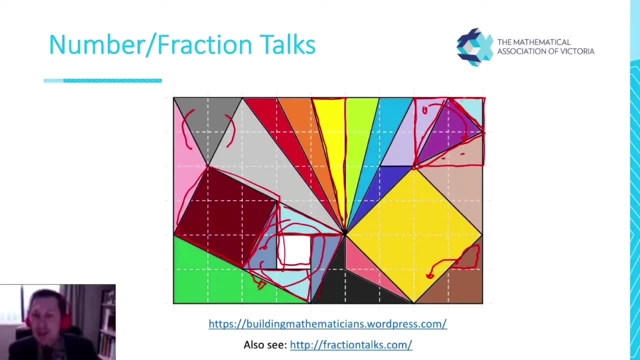 Yep, then take away that top corner, Then take away the top corner, So you're going four subtract two subtract another half will then get us this part here, the purple one, which would be, of course, one and a half. 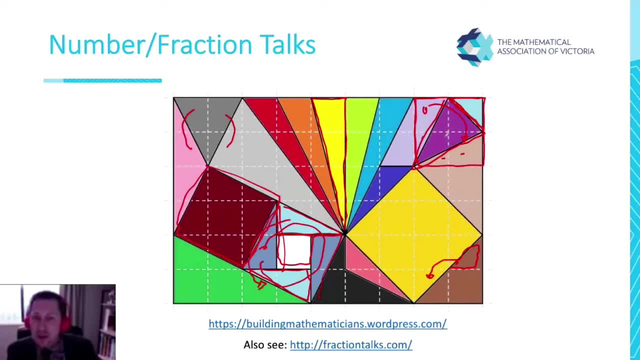 That way and also just rotate the two smaller bottom purple sections to complete the one, The one in the bottom left corner. Oh, I like that. So you're saying if I got this part here and I move that around to there, and if I got this part here and I move that around to here? 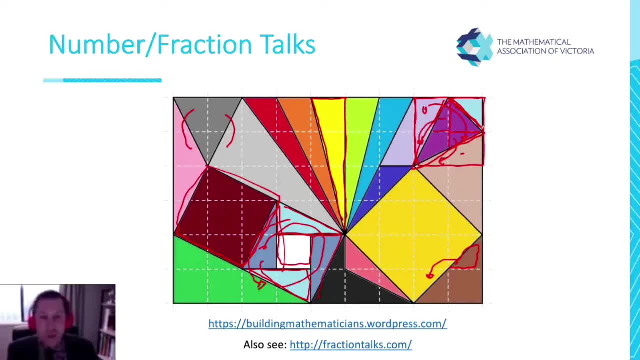 Yeah, And that would make my one, and then I've got my one half there, Oh nice, I really like that. All right, this is the whole point And this is what I mean in terms of fun When I first came up- and maybe it's just me, maybe I'm just one of those- 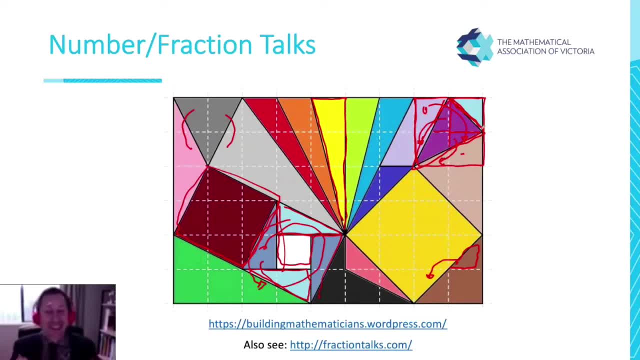 those people that just get excited by colours, pretty colours and bright lights. In fact, I am one of those people, But when it when it came to this, I saw it and I just went. I found myself spending the next five minutes going. 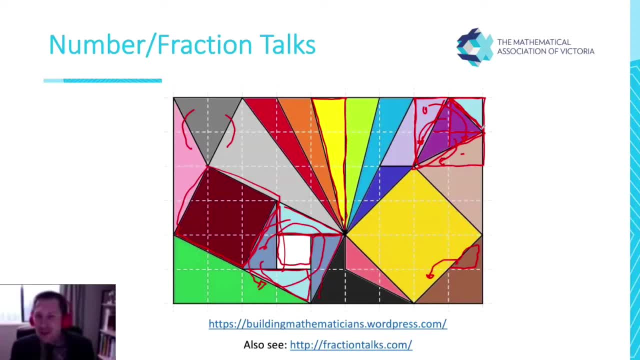 Oh, what's this one equal? And trying to figure my way through and nut them out- And there's always ones like this purple one that you could see here- that really stood out to me, And this is what I mean in terms of mathematical reasoning, is fun. 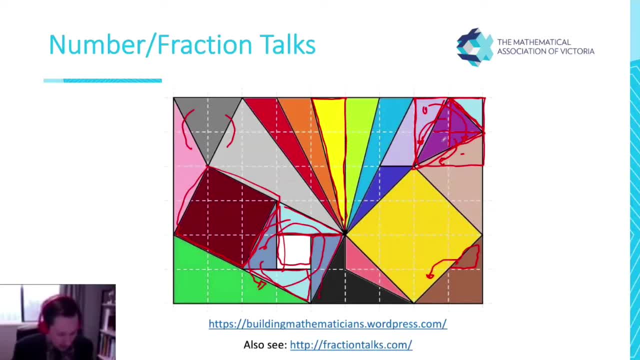 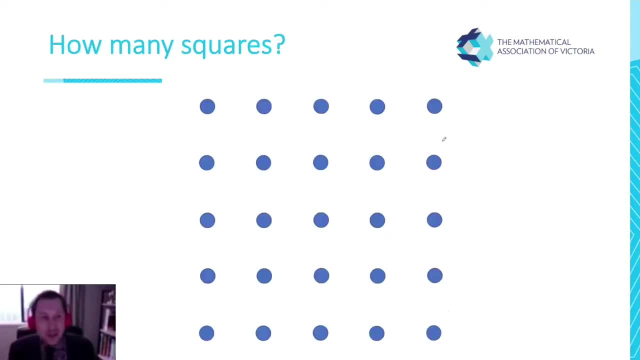 All right, This is, and this is why I see it as being fun. I'm just going to go, I'm just going to remove this stuff up here and we'll go to the next one. Another task Let's see I've got in terms of mathematical reasoning is what you've got here. 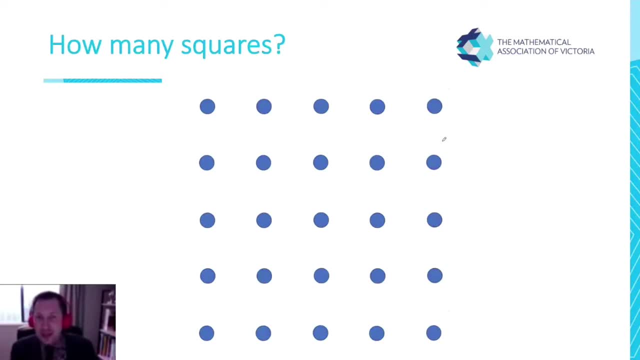 is: how many squares can you make on this using this here? Now I'm actually going to copy the links in. I'll go command V: If you go to the first link that you can see on the screen, Okay, Uh, the first link that you see on the screen, you'll see it's going to take you to. 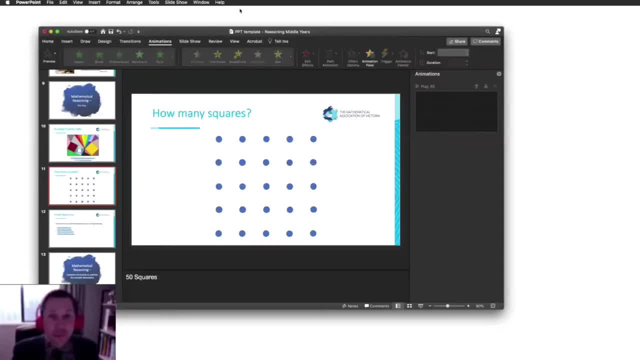 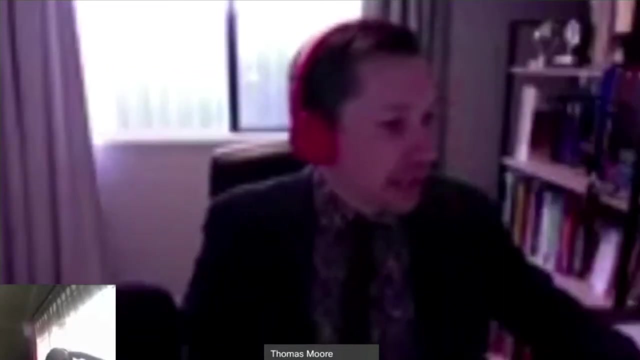 I'll share my other screen with you. Um, you'll see, it's going to You, to. I'm just going to get to the right part, Okay, So hopefully we can all say that now, You'll see, you'll take you to this. 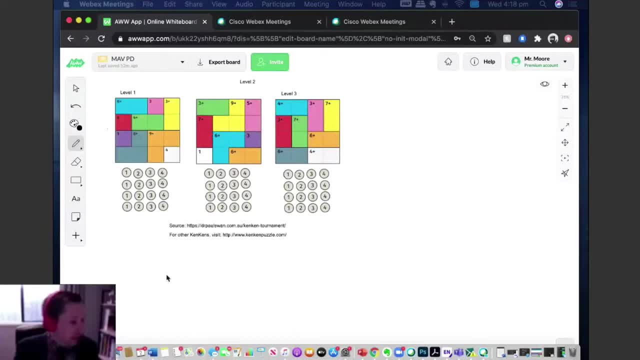 Now what you can do is you can come down to the bottom part of this screen here, and you'll see that there's another um, another arrow, or an arrow that will take you to the next part. This will bring you To your foot. your dots there. 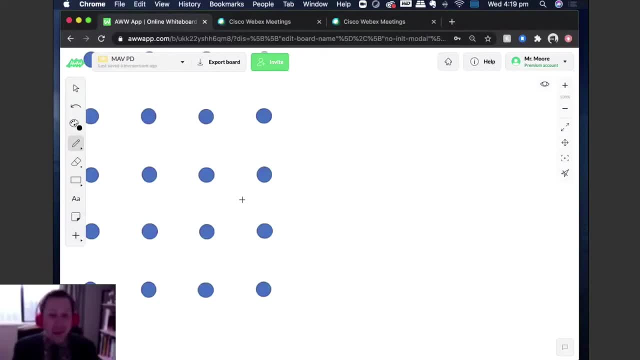 So you can have a play around with it. I'm interested to know how many squares can you make on this actual screen. So have a play around with it for the next couple of minutes and see how many you can find. Feel free to put it in the chat. 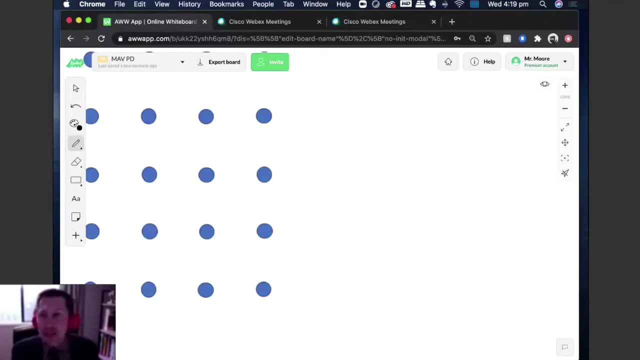 Once you've found out or once you think you've got the answer. Okay, I've got a couple of people. go on 30, Michael, would you? oh, okay, So Michael said 30 and then he's retracted that. 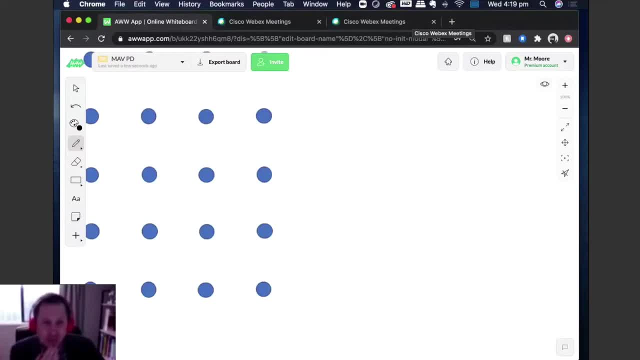 Now I've got Alan or so, and and Hong is saying: Hong saying more than 30. Michael, could you share what you're thinking is when you saying retract 30. Well, can you hear me? Um, yes, I can hear you. 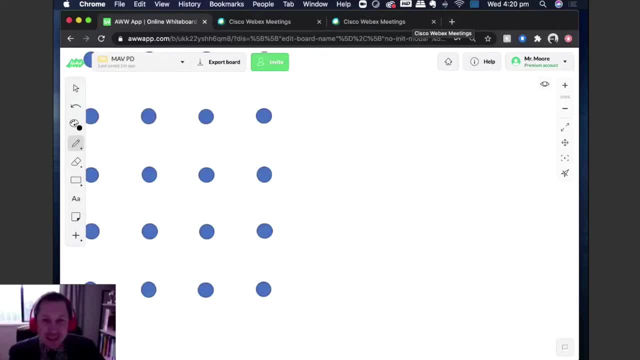 I originally thought 30, based on the squares That are based on vertical and horizontal lines, but then have realized there's also squares that are orientated diagonally. Ah, so you're saying you can rotate the square, So a square is still a square. 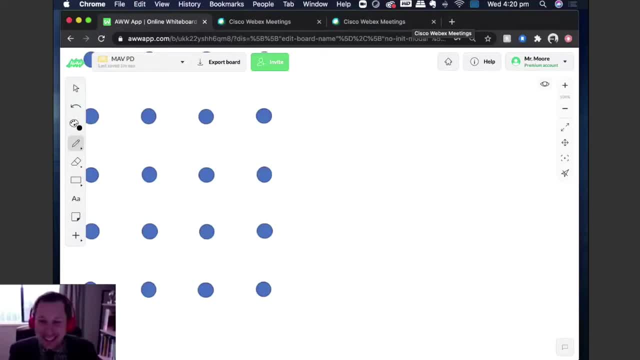 If you rotate it. Yes, Yeah, Nice, Okay, Awesome, All right, Well then I'll leave you guys to have a bit of a play around with it. So let's see how many we can find there and think about as you're doing this. 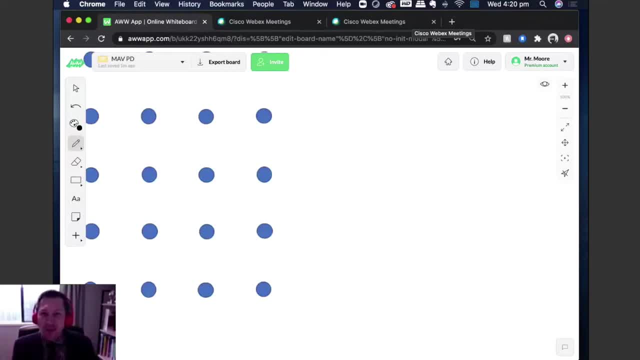 the process, the muddling that you're going through in order to be able to find them all. Okay. Okay, Then let's take a look at the next slide. So we have a lot of bright dots on the back of you here. 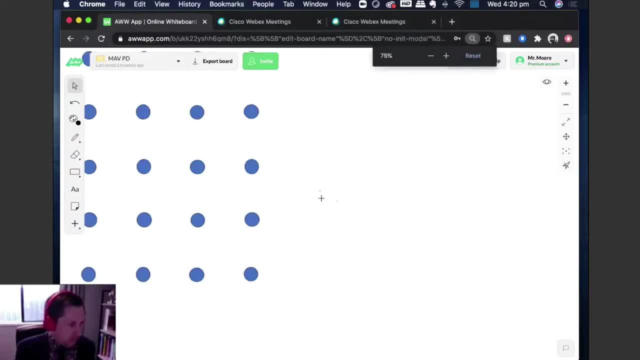 so for this to be, this is kind of an exercise. you're gonna have to make a lot of different variations. I mean, it's not gonna be that different for you to be able to understand them all at the same time, and maybe you're not gonna be able to figure them out. 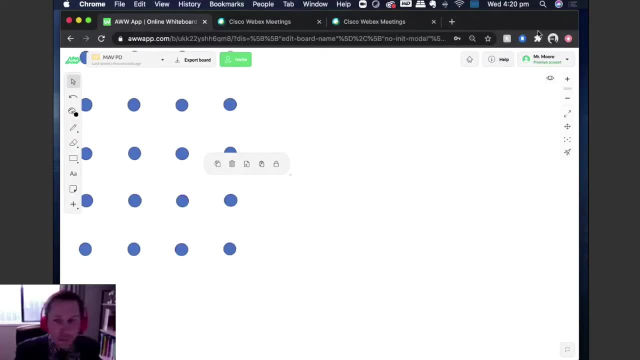 at the same time, So you can make something out of them. And if you think you can't with another answer, feel free to put it into the chat as well. Also, I've tried to figure out how to move all my screen around. 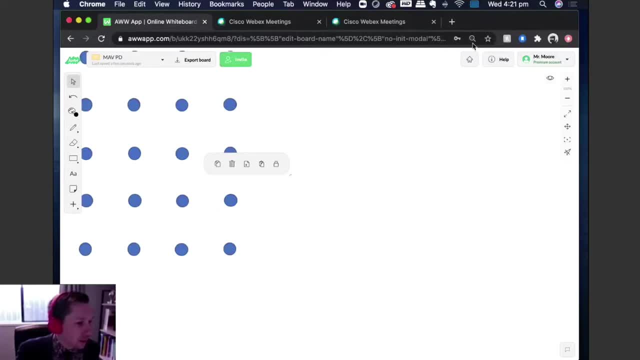 okay, so what Michael was saying before was: obviously, a square is still a square if we rotate it. so I mean, that's a terrible attempt at a square, but you get the idea if I rotate it around. so. so there's more than the the normal thing that we would lay out. okay, so now we're getting up to 42. 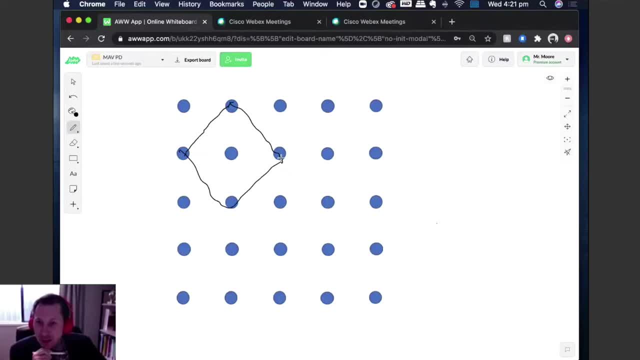 and 40. are there more? because that's the thing is: once we start to get to the point where we think we've got them, it's now a matter of making sure that we're 100, sure that there's actually 40, so are there, in fact, more? 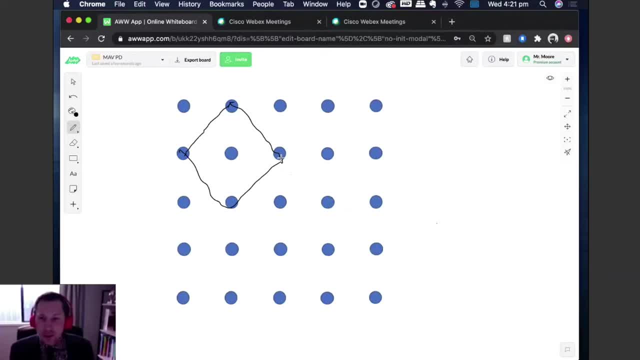 so Simon's saying 25, or 25 factorial, which 25 factorial will be a lot um, or is he saying 25? so what is it? i can see jody's got a 42. oh okay, prather's saying you could also have squares which are tilted at 60 degrees, and what? 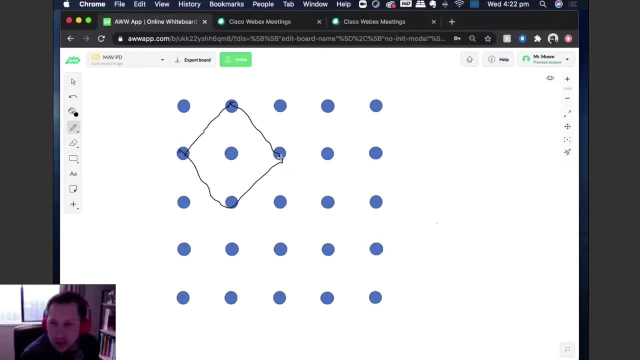 about overlay. so so i guess, for example, in terms of asking the overlay stuff, this here is still another square, you can still make another square using that, but you've got one square here, you got the one square that we've got here, and then we've got another square, that's over. 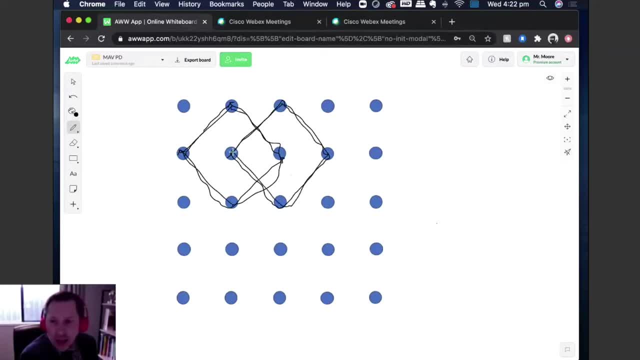 the top of that. so that's, that's two squares. so you can have ones which overlay, but obviously you can't have ones which go directly on top. for example, if i did one square here and then another one straight on top of that, that's the same square. 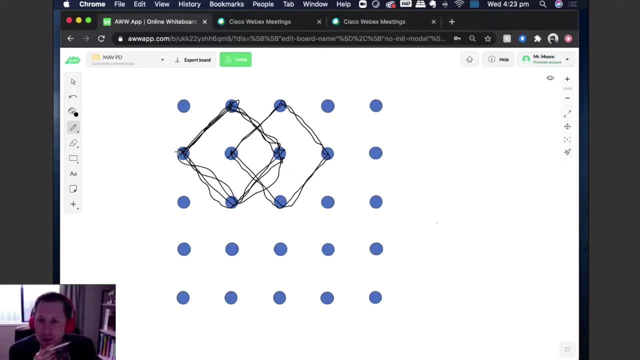 so, um, probably not then the, then the square in the middle there. oh no, no, i got what you're saying now, sally. so with the square in particular, it's got to be sort of the ones that it's like on a geo board. if you had a rubber band and you put a rubber band around the geo board, how would you? 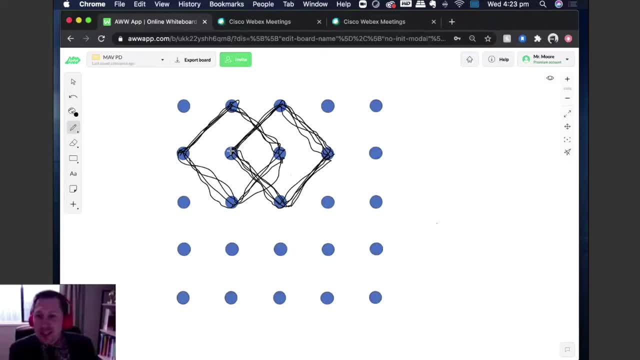 make those squares? great question. so, yes, they need to go through the dots. great point. all right, so i can see. can we see, as we're going through this, some of the reasoning that is coming through? oh, michael's now caught with 56, so we're now getting more and more, aren't we? 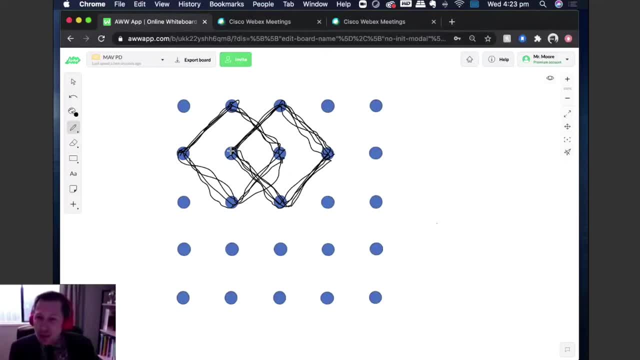 the challenge now. and what about overlays of different dimensions? haha, now we're talking. now we're talking about things like real mathematical reasoning, so we're taking things further. so once we, once we've got all of them, and we know we've got all of them and that goes. 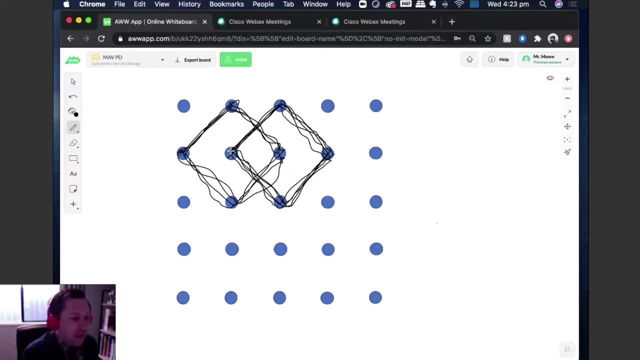 through the reasoning process you might start to think: okay, well, what happens if i then add other dimensions? so maybe what happens if i had a five by six or a six by six? what happens if i did the square from overlapping um structures? you know what could happen there. there is so much that 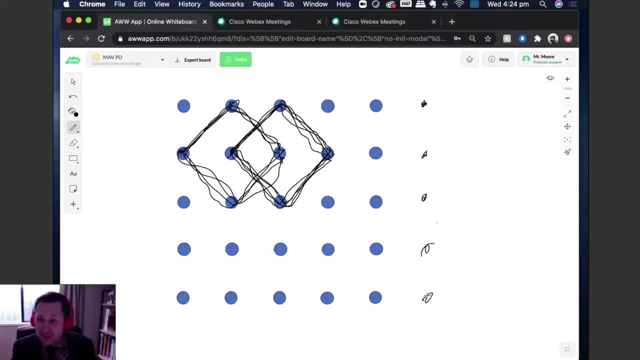 could be explored in this. prathu's saying that there's 50.. all right, there's. so we're now starting to get to a point where we could really go through and explore it more. xavier is saying 50 as well. so prathu and xavier both saying 50, ruth saying 56. we've got a whole lot of different answers coming. 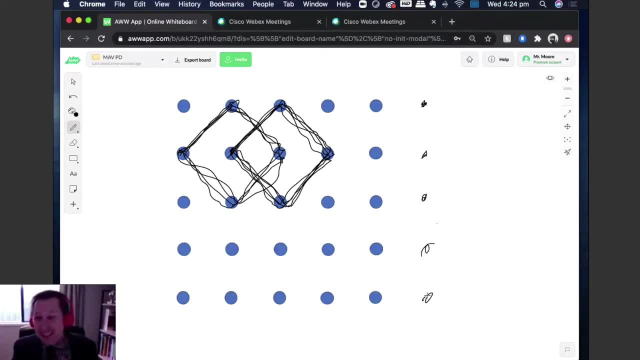 through right now, which which is really cool. now i'm not going to actually tell you the answer. i'd love for you to go through the answer, but i'm not going to tell you the answer. i'd love for you to go and explore it, because then, as soon as i give you the answer, when it comes to mathematical reasoning, 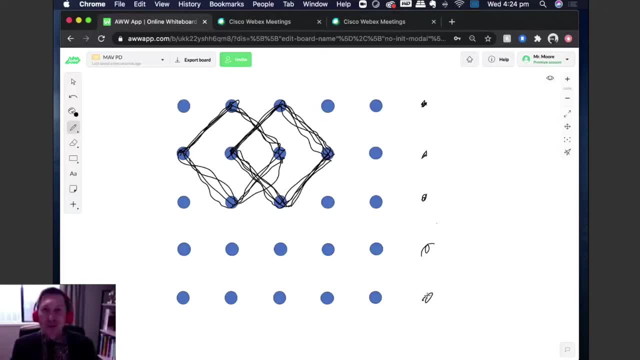 i've taken away all the fun. hopefully, at this point, what you're noticing is this, this investment. like i said, mathematical reasoning is like it's the hero on the plate, it's the chunky bit that you want to stick your teeth into and just have a go at. that's the stuff. and as soon as i tell you what, 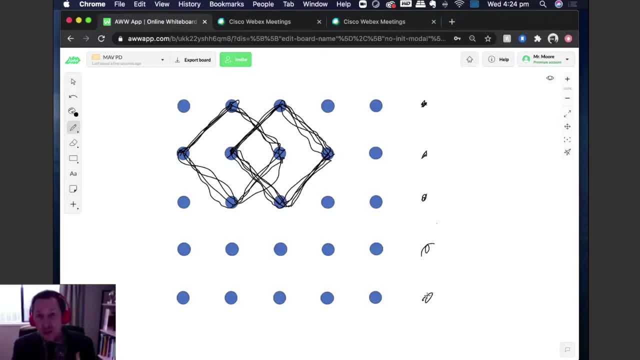 the answer is that kind of removes it for you, especially if you're trying to work through it. so it's about going through and trying to figure out and know that you've got them all, and do that in a way that makes sense. so i'm sorry if i didn't get it. i'm sorry if i didn't get it. i'm sorry if i. 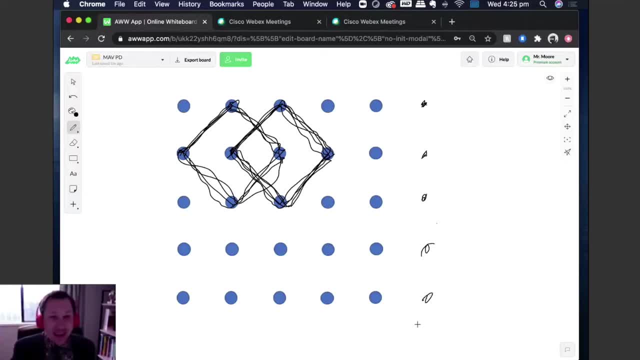 didn't get it. i'm sorry, but i'm not going to give you the answer today. all right, i'm going to bring it back um to the next part of the presentation, because we're going to spend the next half an hour talking about another part of mathematical reasoning that i think is important, so bear with. 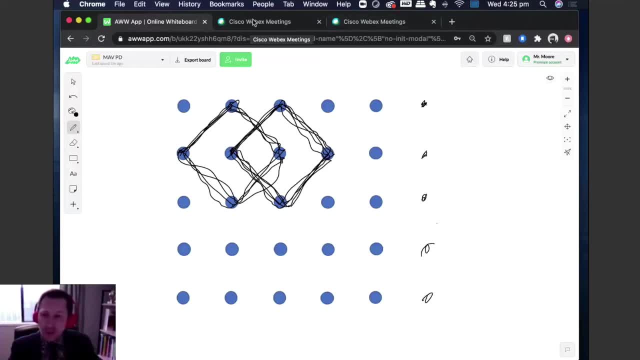 me a second whilst i get my screen up and running. if you want, feel free to have a go at still doing this whilst i do it. would some students engage better with finding the different sizes and orientations rather than just the final number? maybe, maybe, absolutely, and so you've got to this. 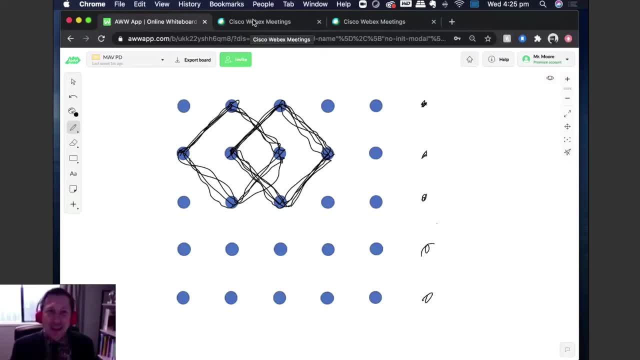 is part of the agency with students, isn't it? you know, if we can allow them to have the opportunity to go off and explore a particular thing that they're interested in, are they still working mathematically? are they still reasoning? absolutely so. that's probably the goal, or the learning. 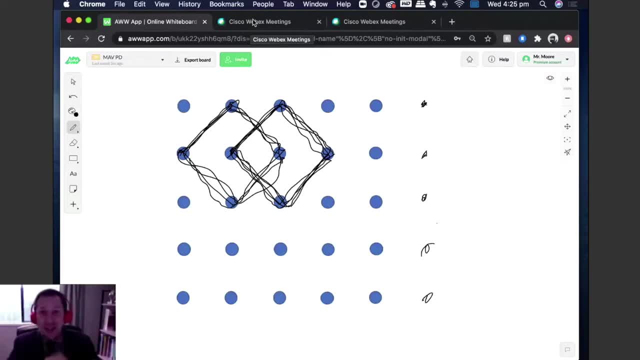 intention or the goal that i would have for the lesson is: are students doing this? are they? are they reasoning? are they working mathematically? and if they are, doesn't matter how they're going about doing it. they don't have to answer our question that we put out to them. they can answer. 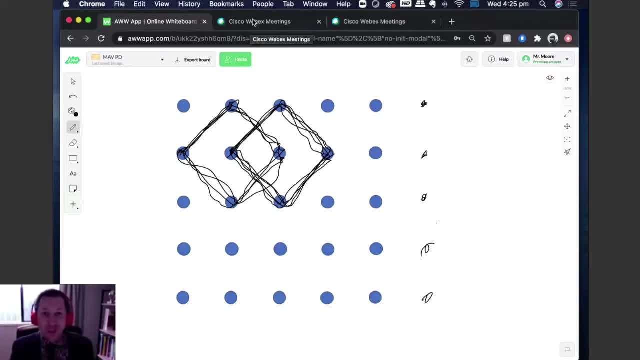 their own question, and and we should encourage that more, because the more we do that, the more students will see mathematics as being something that's a creative endeavor, rather than something that we just force down their throats, which, um, you know we don't want to do, but at times that students can perceive it that way, so awesome. feel free to put all the other. 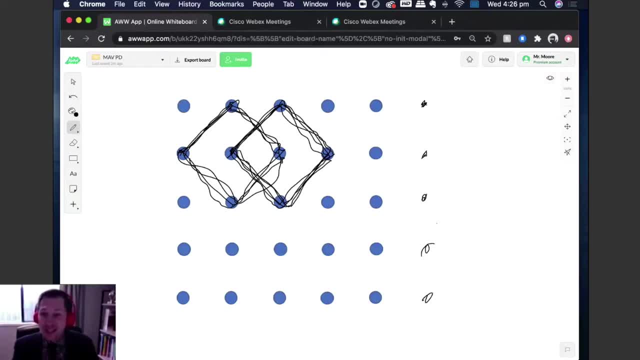 adaptions and stuff that you could see in here. i'm loving some of the chat, so from from um daniella, like: how many, what are the number of rectangles and all that kind of thing- triangles? feel free to put other adaptions in here whilst i thought out my screen. uh, i will try and do that now. 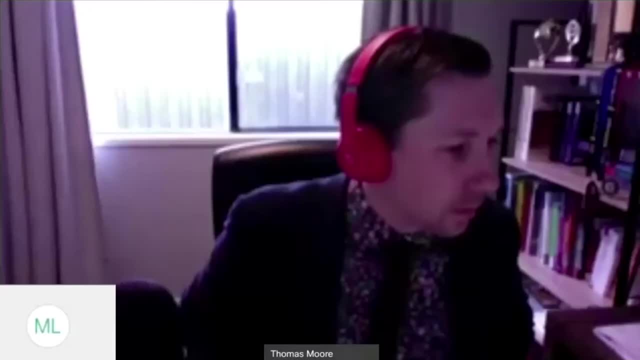 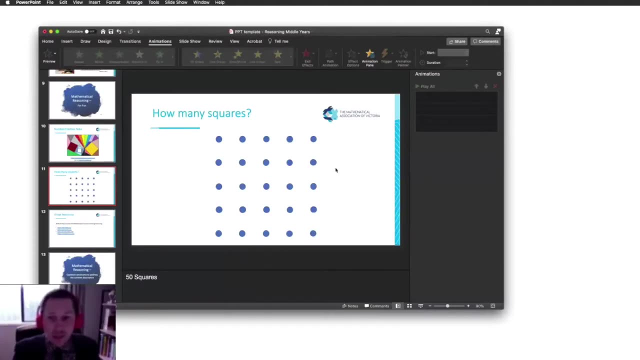 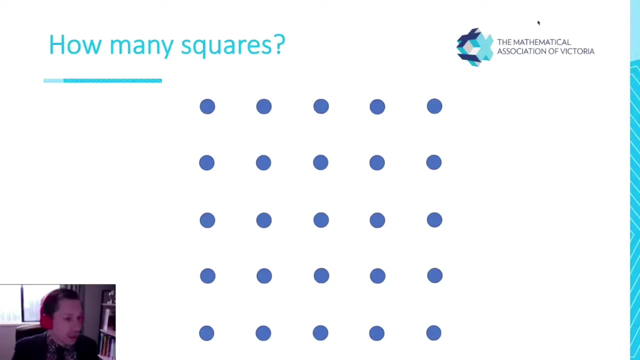 okay, so we should be seeing my powerpoint screen again. uh, and i'll bring this up here. okay, bear with me. last couple seconds now. can i just get confirmed that people are able to see my powerpoint screen as well? just also whilst i'm looking at the chat. 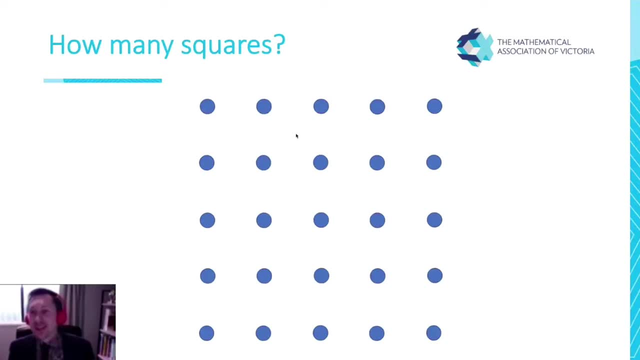 yes, thank you very much and awesome. thank you so much for that. so i love as well all these different ideas in terms of taking it further. is there a rule that you can find? um, so that you know, if you know the dimensions on the dot grid, you'll know the squares right away. wow, what a great. 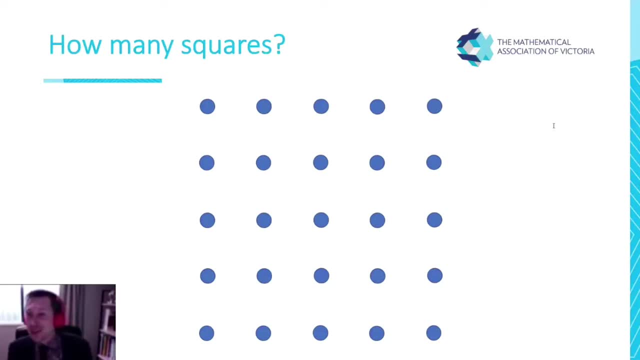 generalization- kind of thing that you could go through and do. my mentor once told me that a student thinking about their subject and the applications of what of it whilst at work or sport was just as valuable as them completing the practice questions. yeah, absolutely, absolutely. thank you for sharing that. 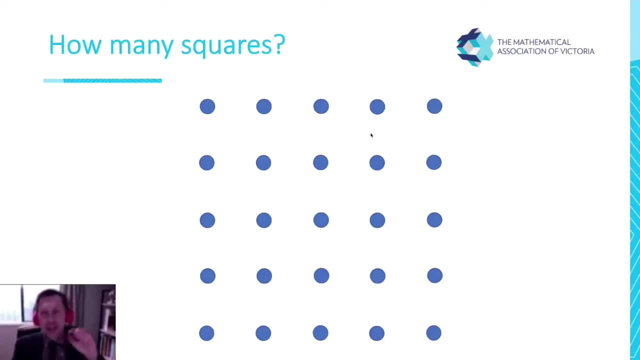 all right, let's go through. and so these ones, these are the kind of tasks that i could do all day long and and we could really go and explore and pull them apart. and in fact, there's a great group of people um mass teacher circles, which i highly recommend people look them up on. 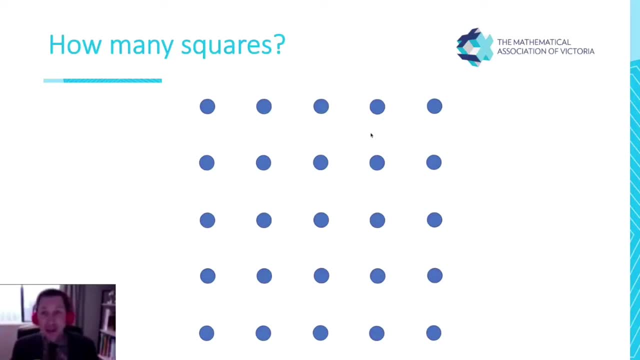 facebook. um, and it's run by michaela evstein and alex box, who i believe we've got alex with us today. um, they, they run this pd for teachers and it's really cheap. it's, um, if you're a member of mass teacher circles, it's five bucks and you go through and you just explore these tasks as a team. 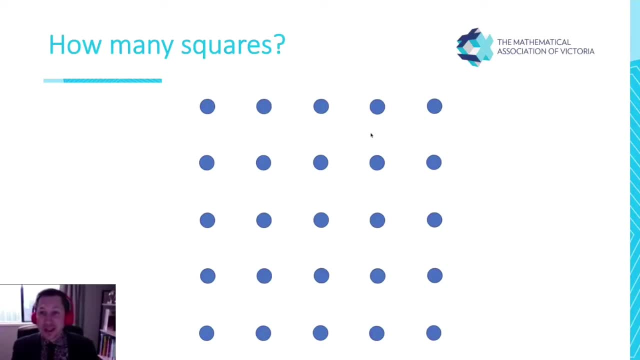 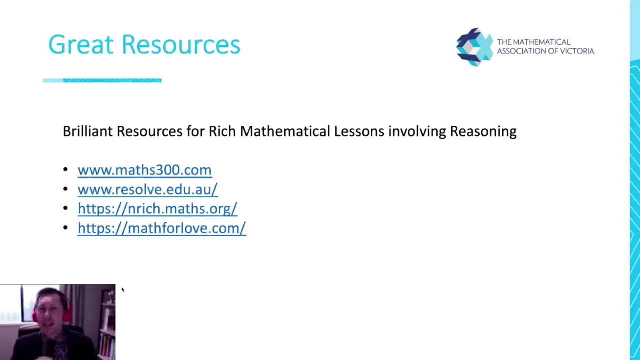 and and really pull them apart and it's really really great. so i highly recommend you. um, you have a look at that stuff. okay, i'm just gonna climb that cool. so next one: these are great resources that you can use for that type of task, the rich, open end of ones that you can explore and you can 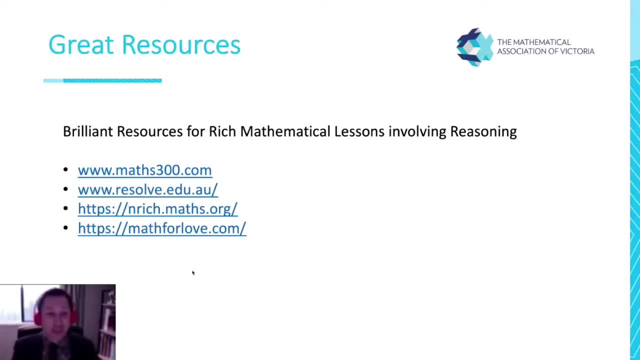 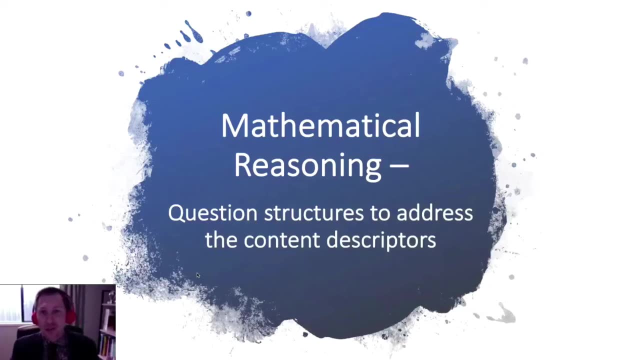 go through and explore these at your own pace. you can spend days looking through all of these um but, but i often get questions ask. the question- and this is a very fair thing- is: you know, that's great, tom, these tasks are absolutely brilliant, but when are we going? 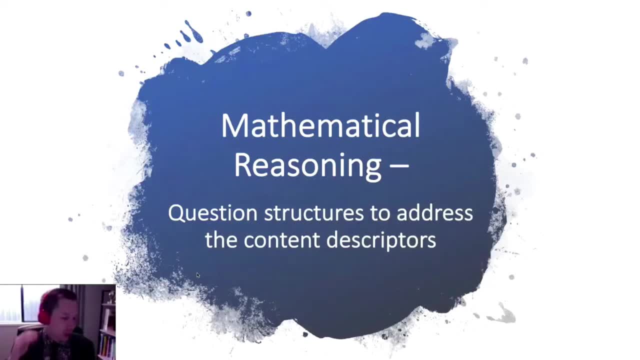 to get to do these with all the other curriculum constraints. you know we've got to get through all these other things. you know how can we actually bring reasoning in? because we just don't have time to do all that stuff and, and, to be honest, like those tasks, i think we need to make time for. 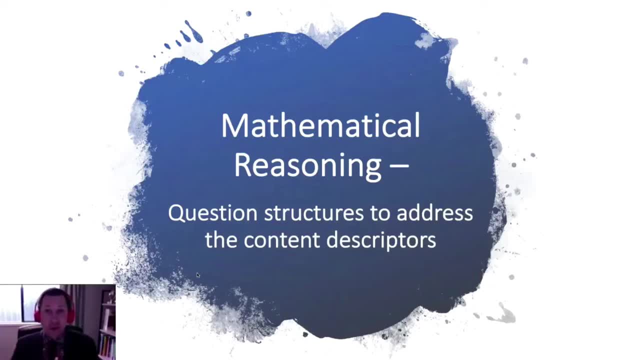 you know it doesn't need to be every lesson by any means, but if we could work on maybe one of those a fortnight at the minimum, that'd be really great for our students. but in saying that, we can still bring reasoning in to our other um into our 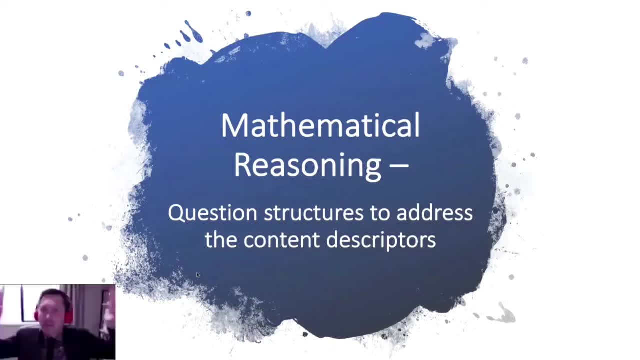 other lessons and this. this is what i'm sort of looking at. so we had reasoning for fun, for the sake of just enjoying maths and experiencing maths. but now we're going to explore some different question structures that you could use in your classes to address the content um. 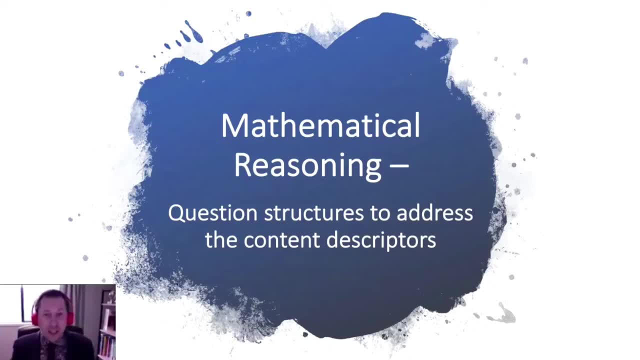 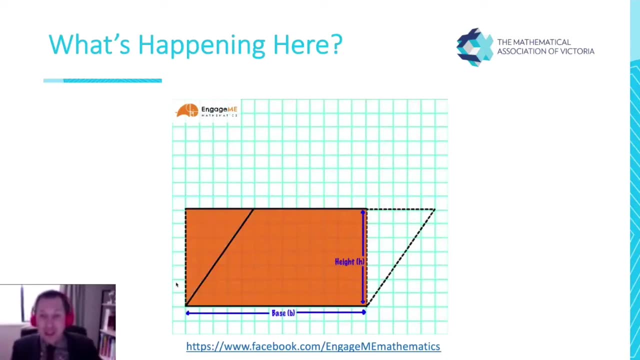 content descriptors that use reasoning. all right, i'll share some of these with you now. if you've seen some of my stuff on engagement mathematics, you'll see. you'll notice that we'll um seen some of these animations, but when the whole purpose of these animations is, i ask the question of students. 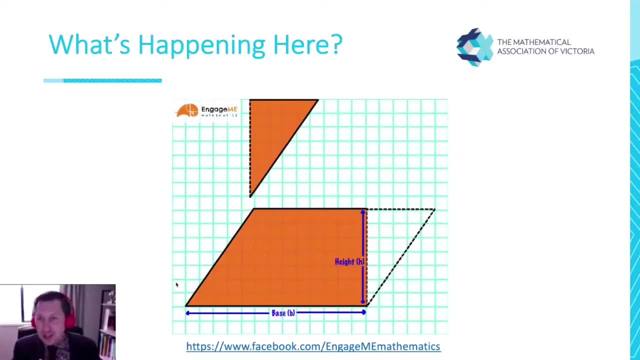 happening here now i'm going to ask you the same question. so have a look through them and, and just feel free, i mean, you, as teachers, will probably be able to pick up pretty quickly. but what is actually happening in this animation? what is it showing us? and thank you, savita, i really 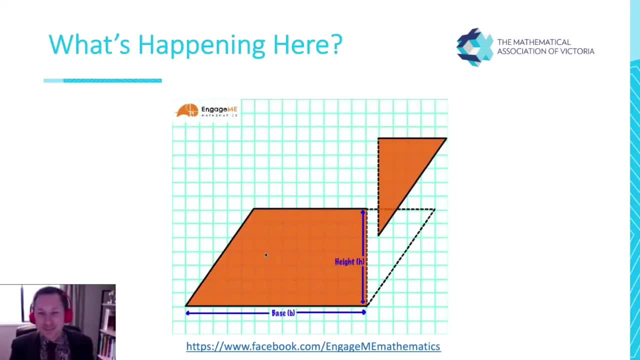 appreciate the feedback on that too. so what is this animation showing us? feel free to put in the chat cool. the area of a parallelogram is equal to the base times the height, or the area of the parallelogram is equal to the same as a rectangle. 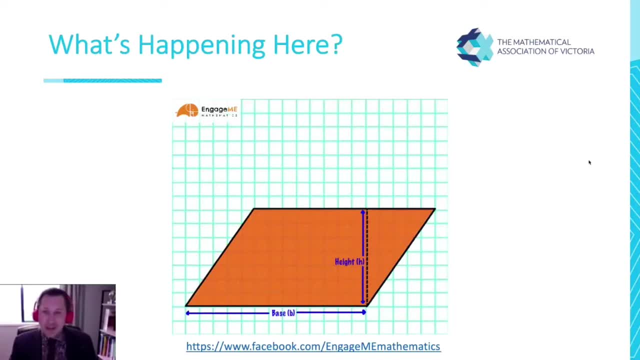 right, so? so just this reason, here we can go: okay, well, i can see what's happening and therefore, if i know the area of a rectangle which most students can figure out because we've worked with arrays and things going through progress, i can then figure out the area of a parallelogram that we 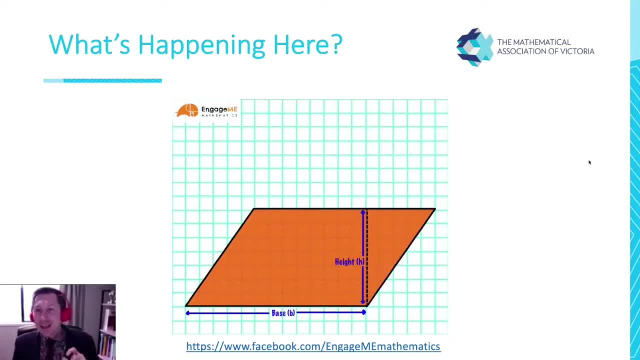 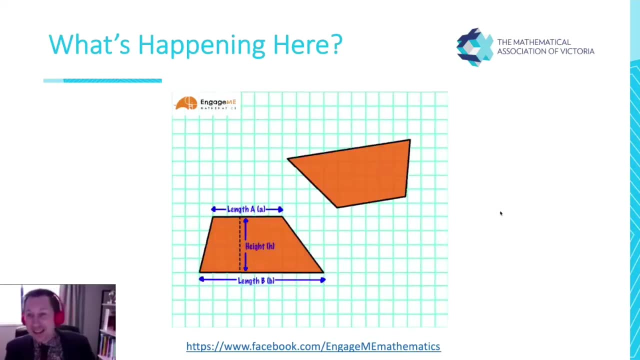 can figure out the area of paragraph using what we know. awesome, now, using this information, let's take it one step further. i'm going to ask you what's happening here and this one. so this is, using this, building on what we've just done one step further. so what's happening here? 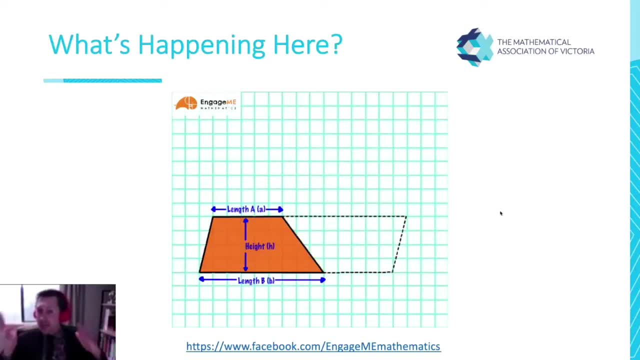 okay. so it's half of a rectangle, because we know it's half of a rectangle because it's half of a parallelogram, don't we? so it's creating a rectangle. that's half of a parallelogram, so it's creating a parallelogram. so two equal trapeziums are equal to one parallelogram. 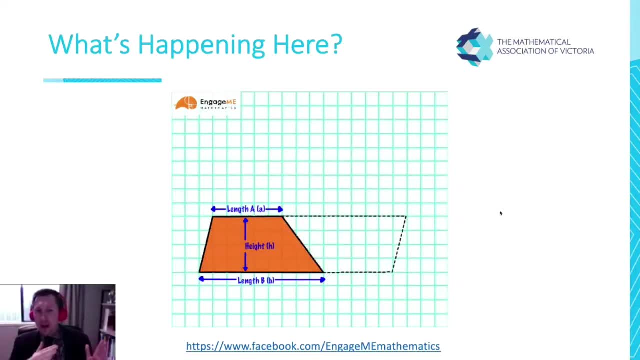 and one trapezium is half a parallelogram. okay, would anyone maybe like to have a go at how we could use this diagram or what's happening here? oh, okay, so now i'm seeing demonstrate: trapezium formula for area shows where the a plus b comes from right. so if we think about this, the, the, 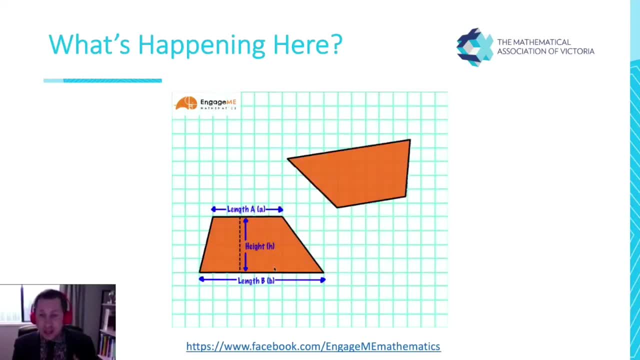 trapezium. the area for a trapezium is the. the formula would actually be, in fact, i'll write it down here: okay, pen. the formula for a trapezium is area equals and it's half of a plus b times the height. now let's just make some sense of this, because i know that this isn't actually. 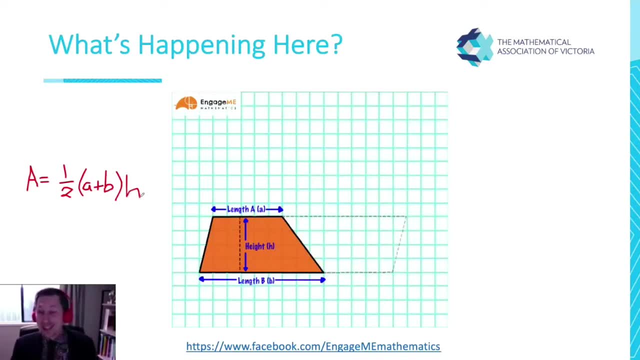 something that i knew off the top of my head when, when i started teaching. in fact, it's not something that i knew off the top of my head when, when i started teaching. in fact, it's took me a good few years before i actually went. oh, that makes sense, and it wasn't until just last. 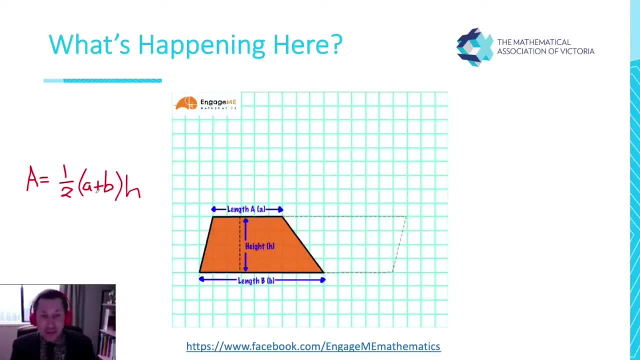 year, that i saw it in terms of what we're looking at now. so let's have a look at this. we know that the base of this parallelogram would be a plus b, because i know that this is b and my a, of course, comes from this part here, doesn't it all right? so now, if i know that, and i know my height well, 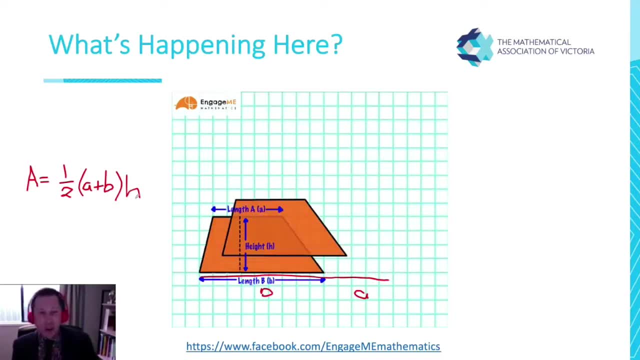 that'll be like saying a plus b times the height will give us the parallelogram, but i only need half of it. so therefore, i've got this here and and i've actually made another one recently where, where it shows the same thing, but using two triangles, for example, you can see here if i drew a triangle going down. 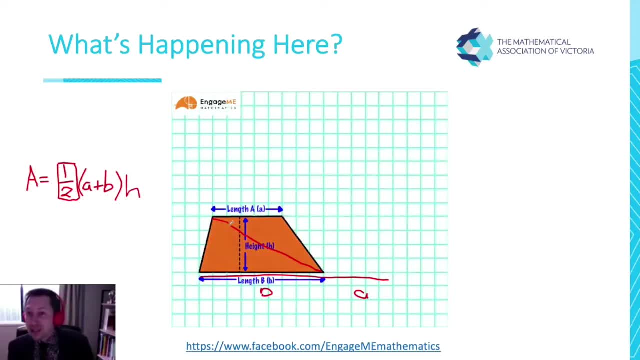 there the same kind of stuff and, awesome, it's got tessellation, so all of these things come through. but the best part about this kind of question that i'm finding is by asking the students what's happening here. what i get is not necessarily always what i want, but it tells me what they do. 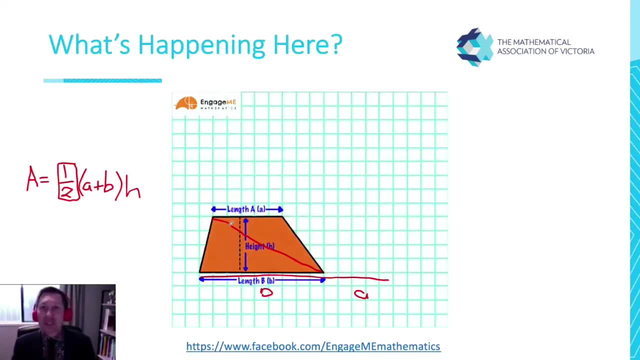 know and it gives me an idea of where i can start focusing my teaching with the students in that lesson. so sometimes it might be taking it a step back, sometimes it might be going okay. i know these kids know a bit about it already so they can go off and do a few more extended kind of questions. 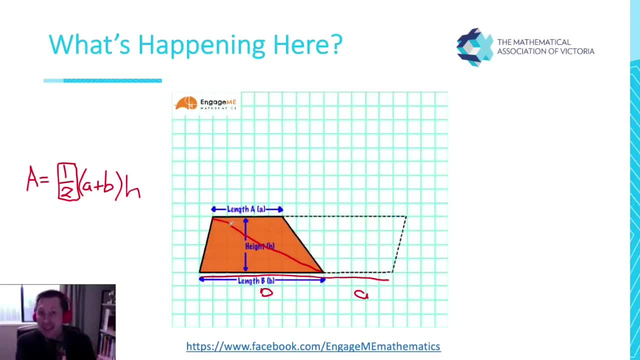 whereas these students probably need to do a bit of work around the formula and understanding how that works too. so it really is a great way of opening up this question. and the other thing is it's sort of like a bit of a challenge. it's a bit of like a secret. hey, can you figure out what's? 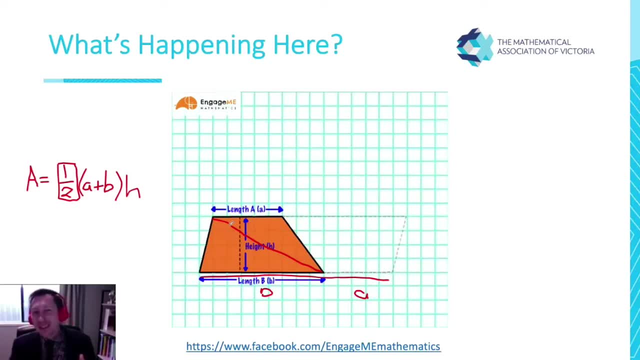 going on here and let them tell us, rather than us just talking to the students and asking them questions, just like i said before, just telling them. it gets them to try and come up with themselves. so let me just, uh, remove this again and i'll go on to the next one, the next one. what's happening here? 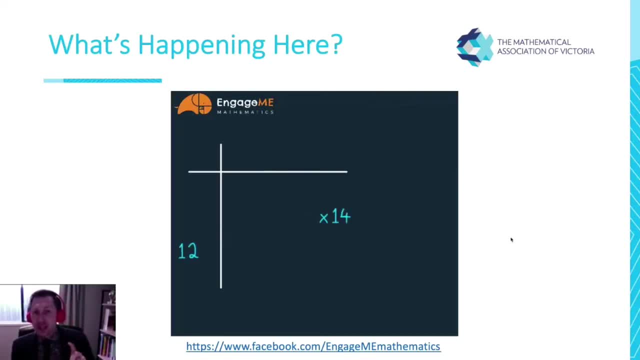 i won't spend too much more time, but i do want to show you two more of these things. i want to put this up, one up here, and i'm going to take it to the next level as well. so have a look at this and just figure out what's happening in this animation. 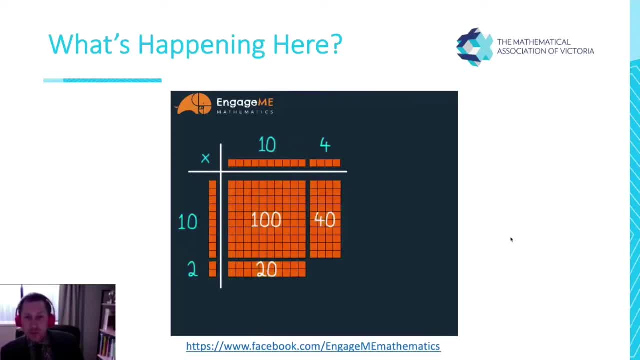 so the first one is the area model. the area model- cool. now some people like will obviously look at this and be like: yep, i can see the area model straight away. the partitioning: yeah, awesome. allison's saying she used it with her grade five. that's brilliant, right. the box method, distributive law: geez, there's so many. 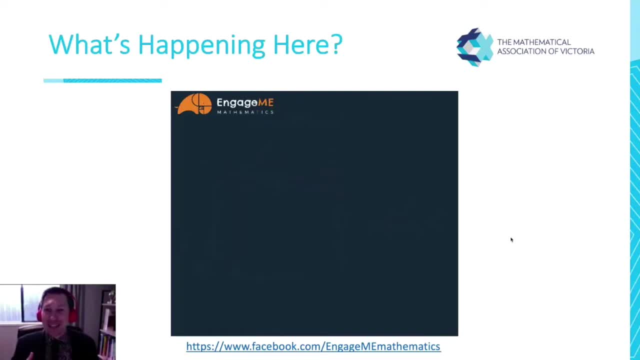 things coming in here. now. we're all talking in terms of, like, what teachers would say and all that kind of thing, but when i showed this one to a year 11 student, it was amazing just seeing the penny drop for them. they went: ah. now I can see how the formula comes about, and what I like to do is 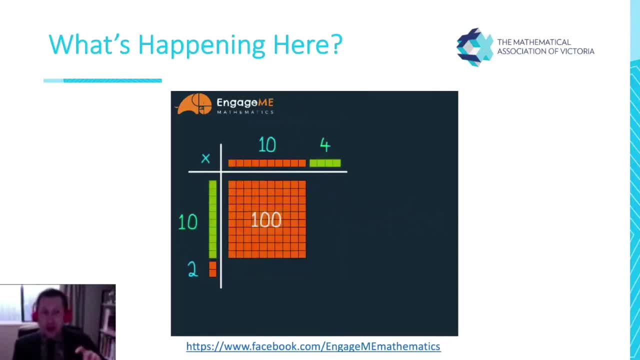 especially for students, once they've seen this and the formula. I would normally start off with this, by the way, but once I've said it, sorry, once students have seen this and the formula, I like to get them to compare the two and see: well, what are? what's actually happening? how does this here relate? 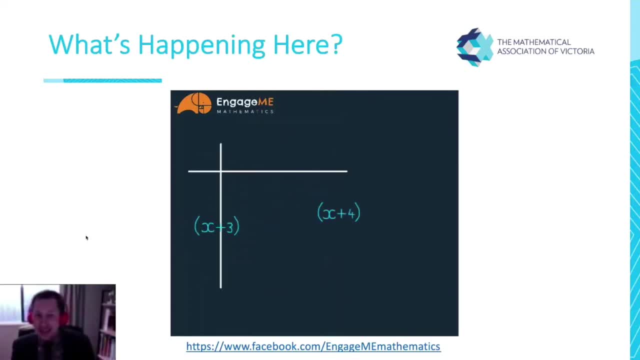 to the formula you might have seen now in saying that we can now see it in terms of another way, and this is for probably for the sake of the primary teachers, looking at: well, why is what you're doing there important for this? all right, so what is happening here? cool. so now? now we've 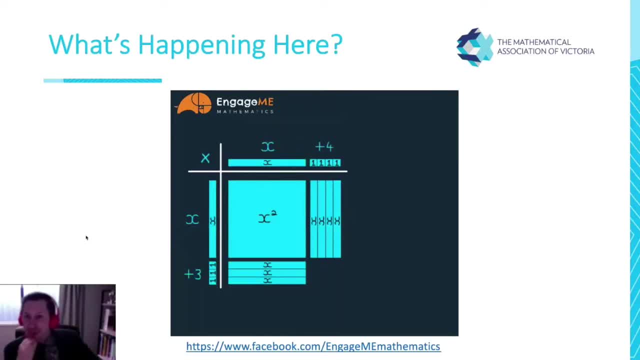 got um. we're now saying so good and hopefully, Nadia, you can see that what you were doing in the with the um, with the primary students five is actually really relevant to to year nine, binomial products and things like that. this is, and this is why it's so important to focus. we can teach. 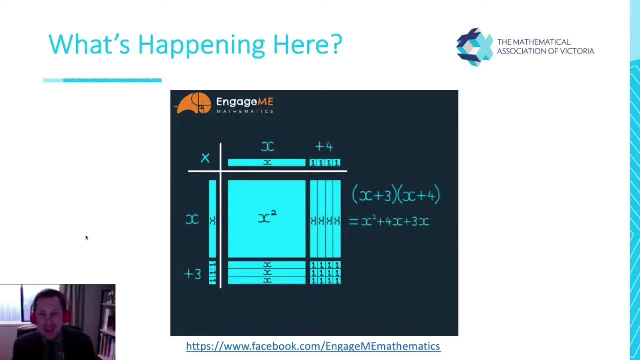 binomial in a way that actually makes sense visually and get them to understand this. now I know, when I ask you guys this question, what's happening here? it's probably quite easy for you to figure out, but when students look at this, there's an element of reasoning and thinking that goes on. that really 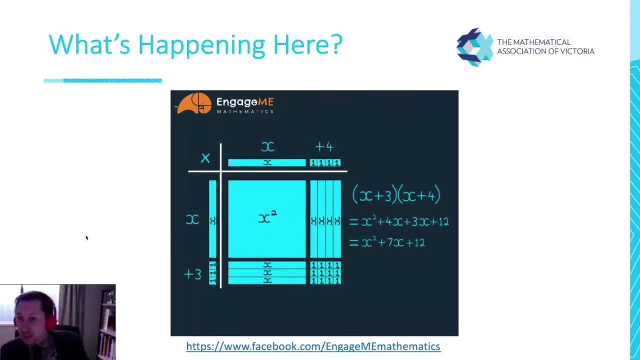 helps out with this. um, massive seed does, yeah, yeah, absolutely. um, it certainly can go up to year 11. in fact, you can use this same model to go through and factorize, and that's one of the animations that I'll get to at some point in time. haven't made one yet about that, but certainly can you. 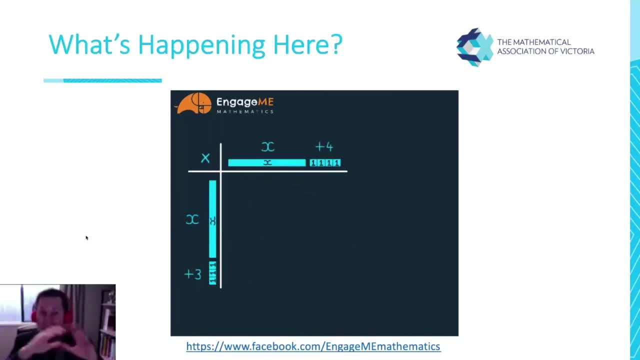 factorize anything for completing the square. there's so much you can do with just using this model and it all starts out with a raise back in primary school. so it's really helpful to go through and and use it and build on all right, and, yeah, that helps with the students to see. 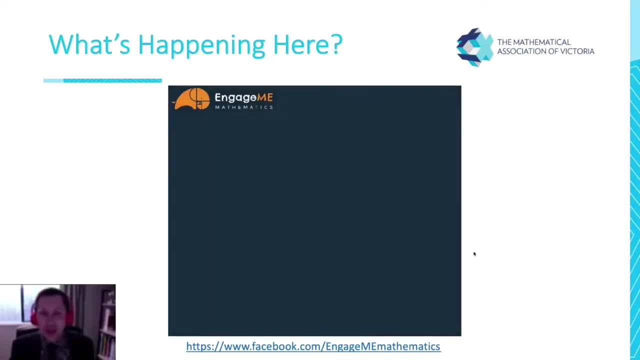 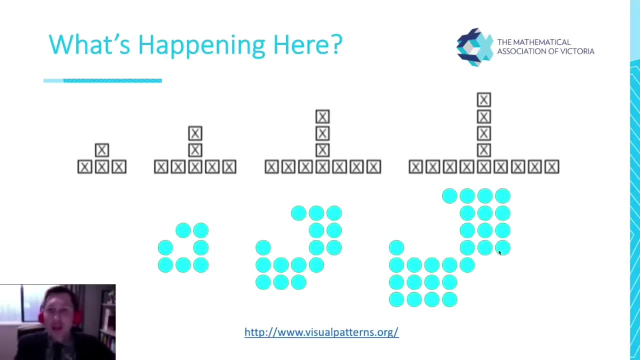 those connections and build those ones in too. so the next one is: I'm just going to have a look at the time here. spare with me a second, because I don't want to go there, we go. so another kind of question that's really um- and this comes from Chris, and I have a question for you, um, and it's a kind of leastPar alley following. how could we have some data put together that would be subjective in these settings? so, and there we go, um. you've got a food and beverage option. that's really um. you've also got this one which is doing that. so if there's um, there's a question: performance. 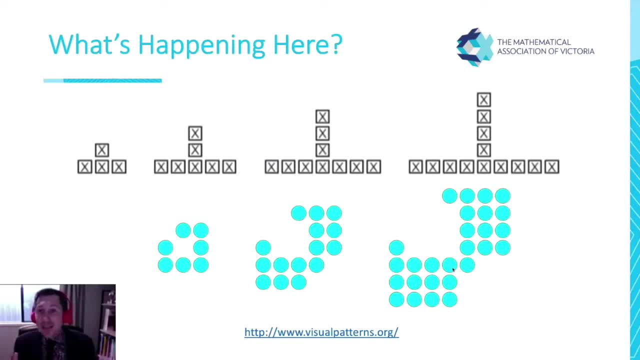 visual patterns is. you know what's happening here and you don't even have to have animations. you could just put up some patterns and ask people what's happening here. so would anyone want to have a go? just put down in the comments, you know what can you see actually happening? how do you? 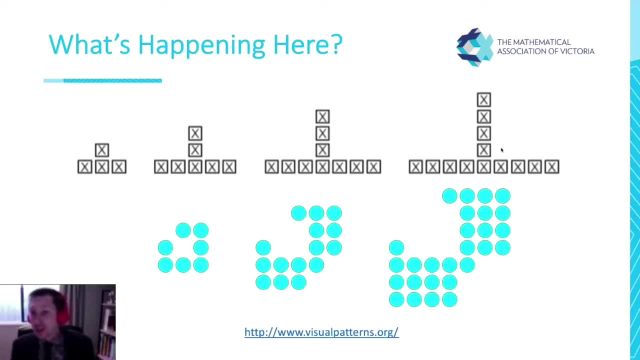 see this growing and if you'd like have a go at maybe what the 10th one would look like. so that's for this is image one at the top. image two on the second one: how do you see it growing and and what would, how many would the tenth have in it? 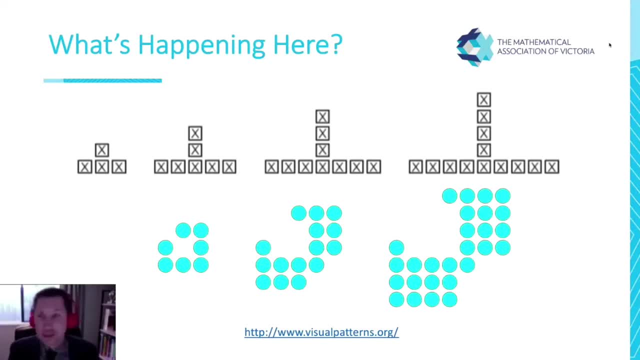 i'll give you a couple of seconds to go through, think about it. put your answers in, okay, so expanding by one on each end. so every time we're sort of putting on an extra one here. awesome, all the three times tables. so is that i assume that that's for the first one, the three times? 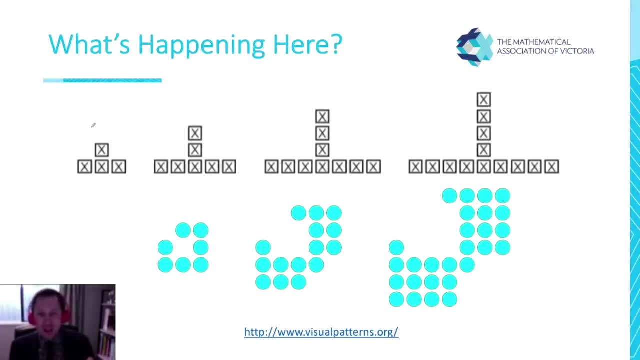 table. now i've deliberately put in one tier that's probably aimed at your, at your grade five kind of thing, and then i've put one that here that's probably aimed at you- year eight, nine sort of thing as well. so 31 for for the n? oh, and okay, i can see 3m plus one. 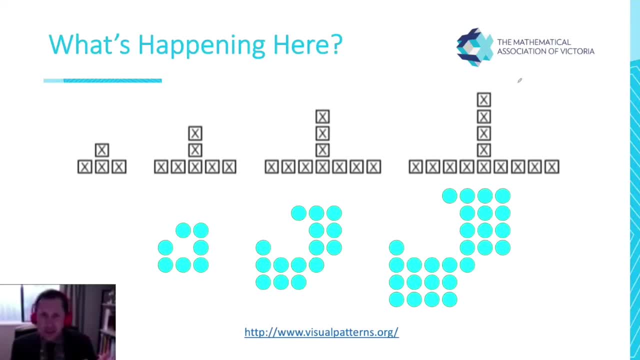 so now we're starting to talk about it in terms of abstractly, in terms of algebra, because we can see, if this here is my third, well, it's kind of saying, well, it's going to be there we go. i've got an n here and then here and then here. so therefore, it's like saying three times three plus one, whereas 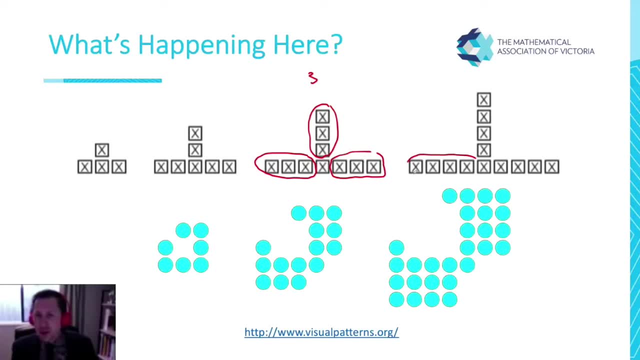 here. well, my n is four, my n is four, my n is four, so that would be like saying three times four plus one. okay, cool. and then if i had ten, if i had ten on this arm, it would be like saying three times ten plus one. so, therefore, that would be thirty one. there might be another way to look at it, though, too. 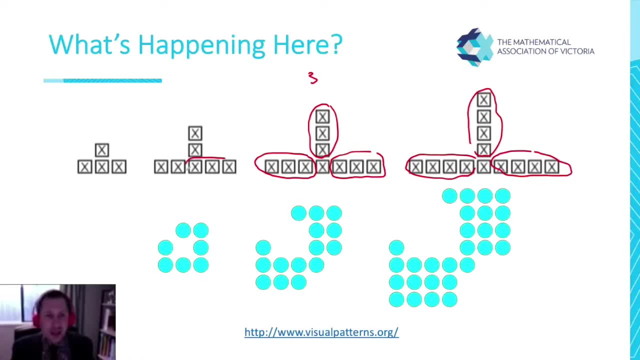 for example, i might see it as being a like this: okay, so in this case that might be two n plus n plus one. can anyone see, can we see, how i've come about that? so that'll be two ends, because that's my second one and i've got an m plus one here, which of course would be three and plus one again. but 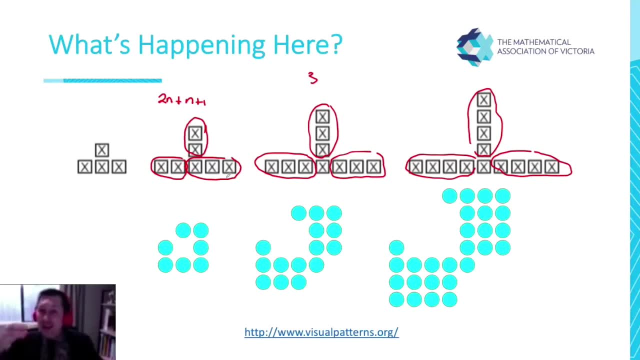 there's different ways that we could go through and see this, and the reasoning is the process of going. once again, it's from looking at this information to taking a step back and going: ah, i can see how all of these connect together. oh cool, jeremy, so you've gone n plus two. n can i get you, jeremy, to jump on the mic? 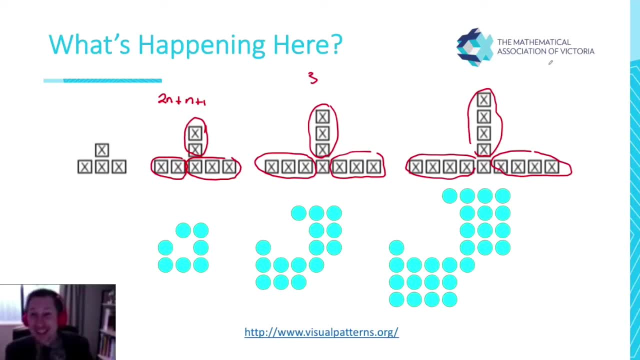 and share your thinking with that, because that sounds exciting. and you're right, barbara. yeah, absolutely. it allows um simplification to discuss simplifying. are you happy to share jeremy? i'm happy to share jeremy. all right, we may move on um. so with this, does anyone, do anyone see what's sort of happening? 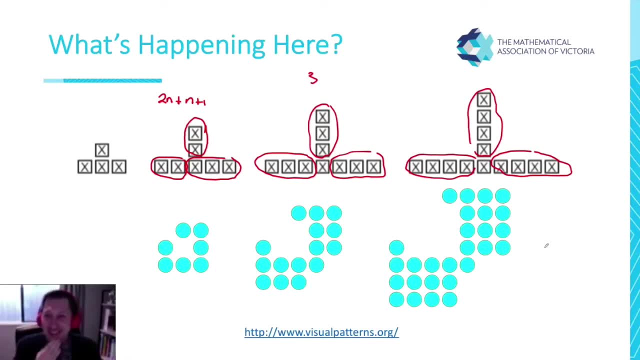 in this bottom one. this one's harder. this one's a fair bit harder. does anyone want to have a go? that's right, thanks, jeremy, i appreciate you. you're sharing your things there, anyway. um so, does anyone want to have a go? what they can see going on in this bottom one, it is a bit harder. 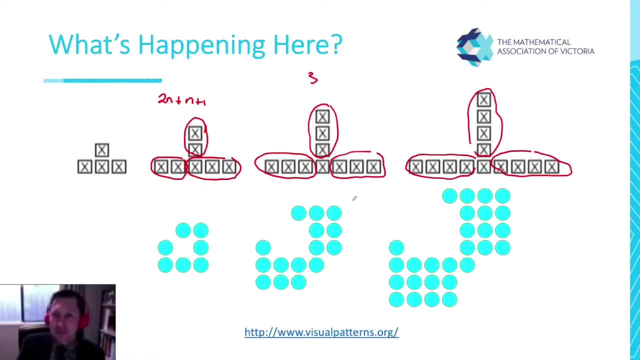 square numbers minus some building in sevens. it's a mirror image, diagonally cool. oh, that's yeah. so now we've got. we've kind of got um, you know, going across the y equals negative x line, kind of thing. there, isn't it? so we've got about um, about symmetry- that's the one that i'm looking for. 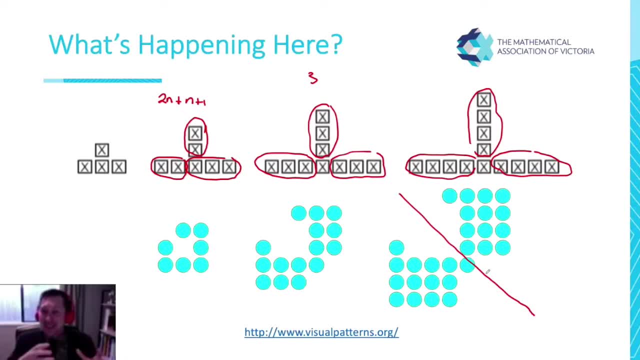 yeah great. so see, even it doesn't, we don't even need to. we can explore in any way we like, but this is when i ask the question: what's happening here? it draws out a whole lot of information. all right, i might share with you how i see it and we'll see if you and i'll share my reasoning. 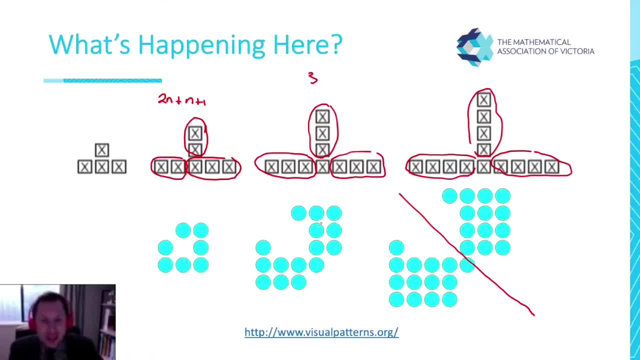 behind it. it's hard to get that from the chats when we're hearing this, but i can. i can see some square numbers coming in here, so, for example, this here is my second and this here is my third, so i'm going to use the numbers two and three in order to do this. ah, now lane's looking at some. 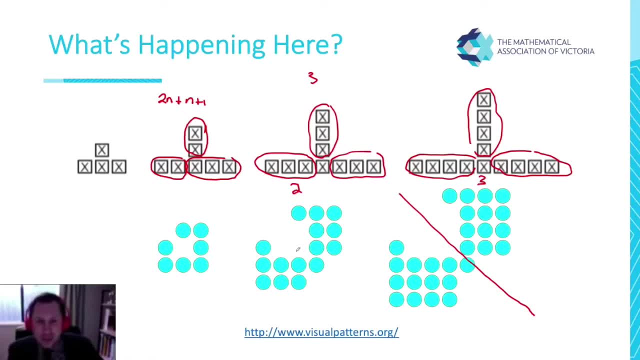 things here as well. so i can see when i do this, i look at maybe a square number here, a two by two, and you can see here that when it goes to three it becomes a three by three, and in fact i can see two of those. so i could see two x squared going on here. all right, because 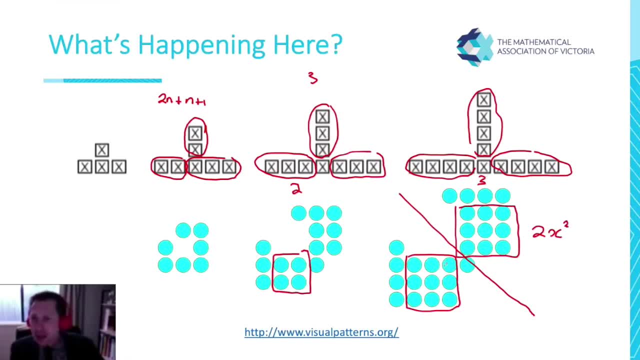 my two squared, my three squared plus. then i can also see: well, here is a an x, because that's a three and that's a three, because. and then we can see: here that's a two and that's a two. so for whatever shape it is, you can see that sort of going on. so so i can see two x's. 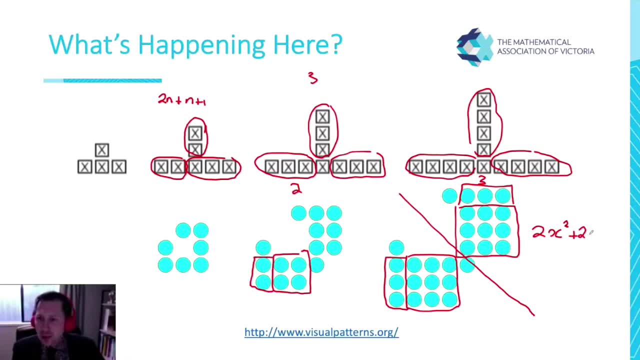 and then i can also see one, two and three, so so plus three now. obviously. i've just gone through and shared that with you and, in fact, if you go through, if you have a look at lanes, what what lanes come up with is most likely going to come out as being the same thing, obviously. 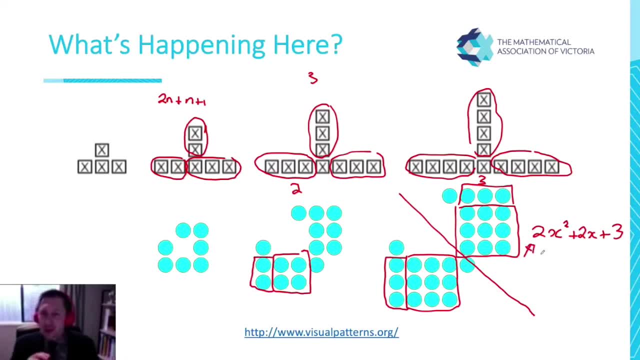 interchanging the ends for x's. hopefully, though, when you, when i went through and demonstrated what i saw, i was able to see that there was a two by two, and i can see that that's a three, and then i can see that there's a two and i can see that that's a three, and i can see that that's a. 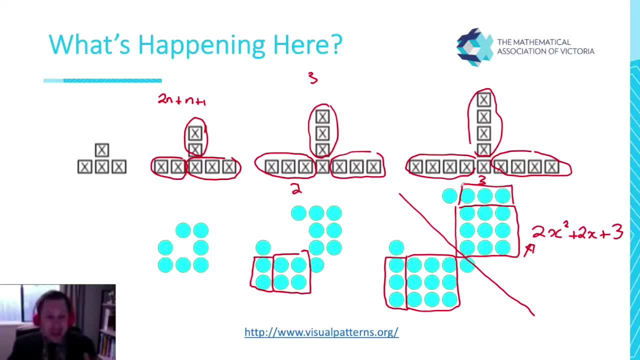 you could see my reasoning and how that came about. and if we can get students to do this, if we can get students to share their reasoning and and make math social and get them to to talk about these things that they can see, then hopefully that'll help other people in the class to be able to. 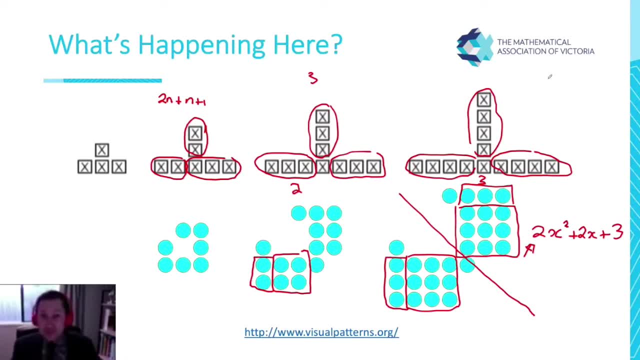 understand where they're coming from. and what would be even better? we don't have time to do it right now, sorry, but if lane shared hers, we could then look at shane lanes and then we could look at: well, how did they, the two, relate, how do they come together? and that once again comes. 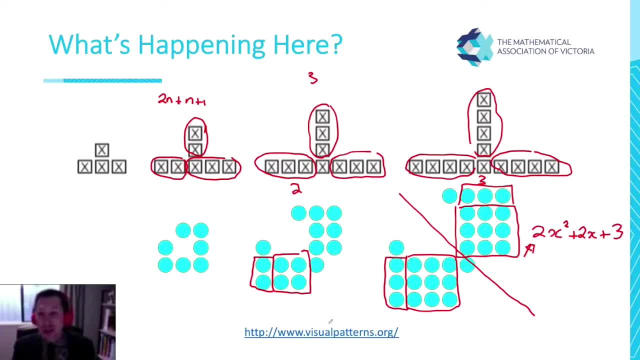 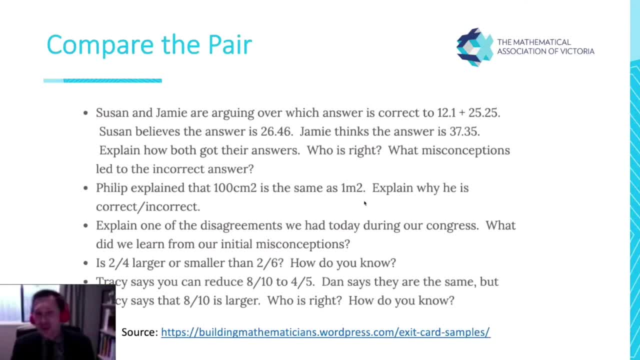 cool and we'll go on to the next page. another, another type of question you can use. so we've looked, we've looked at what's happening. here is a really good way to develop reasoning. another kind of approach that we could use to develop reasoning is a compare the pair like the industry super fund. 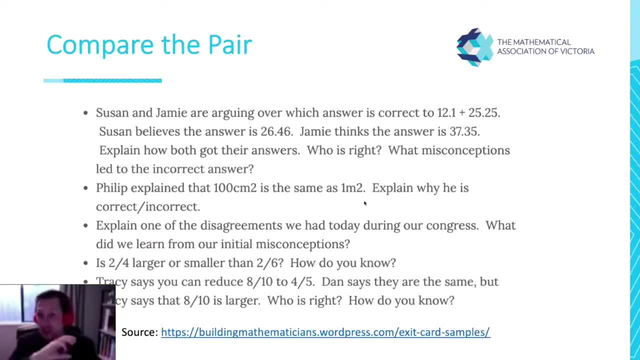 right you can look at, put in a question that is addressing anything you like, like what you can see here, and get students to compare, well, which one's correct, which one's incorrect. how might they got their answers? what might the misconceptions be, and pull apart the answers. 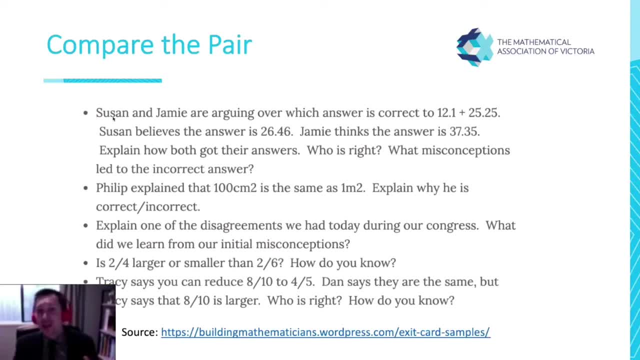 that way, and in fact this here i would argue- if you have one of these kind of questions, you get more from students in doing spending a whole lesson on one of these questions than you would by getting them to do a whole bunch of similar questions that are just the same kind of thing. 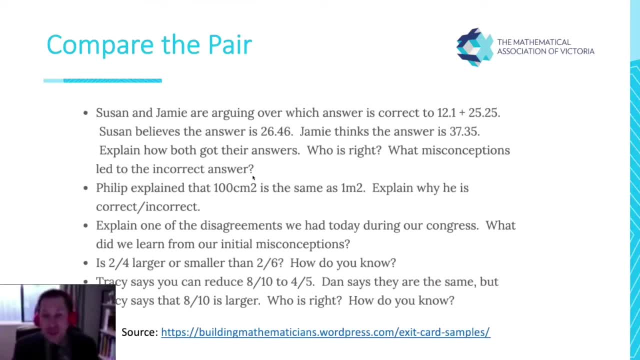 over and over again the reason it comes from. it is really really helpful, um, for both. for both us as teachers to be able to look at- okay, well, this is where our students are thinking at, and then for them to be able to work together as well. all right, uh, is there any one here? 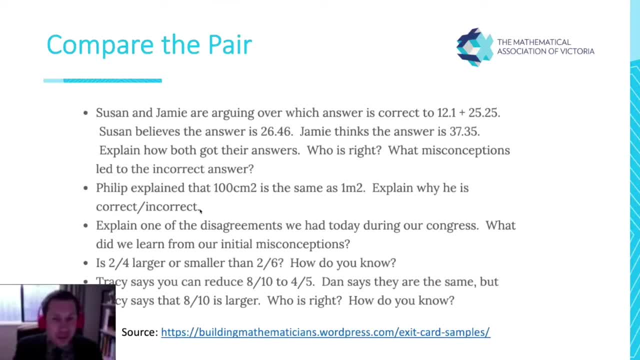 that any one of these questions that stands out to anyone that we'd like to have a look at. philip explained: i, i think i liked, um, i liked actually. let's have a look at this one. tracy says you can reduce 8 tenths to four fifths. 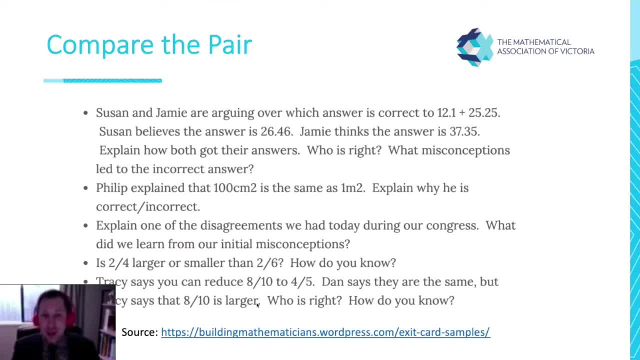 dan says they are the same, but tracy says eight tenths is larger. who is right and how do you know? okay, yeah, so these are great because they address misconceptions. agree entirely. so think about, like as as we read this. a good way to do this is actually to have a think about what. 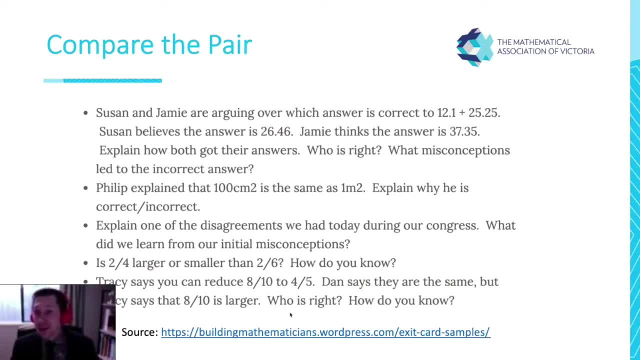 how students might answer it. um, and i really like that one too- the the last one as well, michael, have it like: have a think about how students might answer these questions. so when you look at that- let's have a look at the last one- how do you reckon students might go about answering it? what are the? 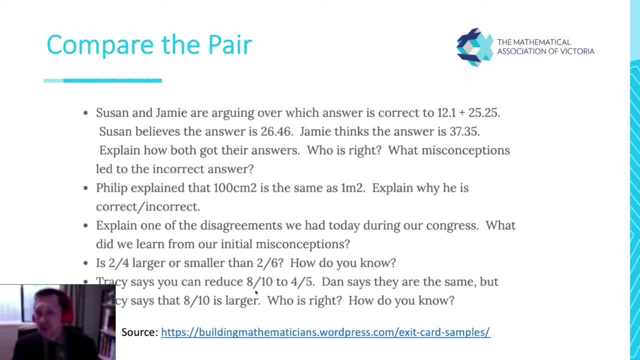 different strategies that they might go to answer this and prove it. all right, feel free to put that in the chat if you have any questions or questions that you would like to have answered in the chat. because, um, so, drawing, drawing, absolutely, i can see students going through and and drawing these. 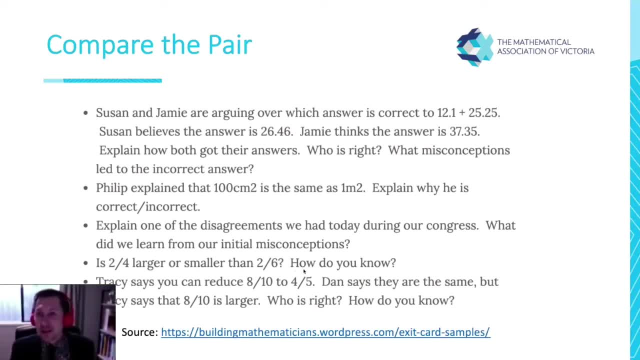 different ways: drawing, paper folding, cool. so we're making a model. we could do that. paper folding drawing- yeah, some students might just. yeah, finding a common multiple: absolutely some students might do that. so there's a whole range of things what i saw. i was working with a teacher who um as part. 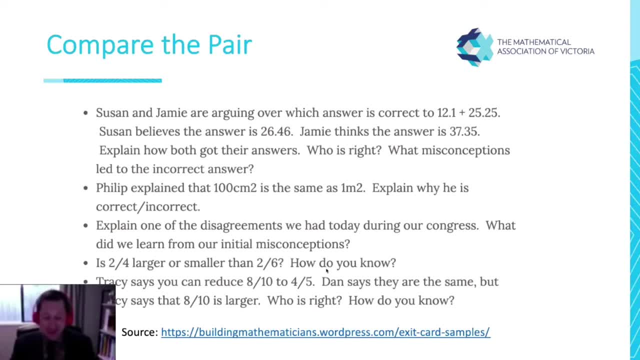 of my research and and short division cool. i was working with a teacher who i was working with a teacher who, as part of my research and what she did was she walked around and took notice of how different people were solving it and then she grouped them according to their strategy and at 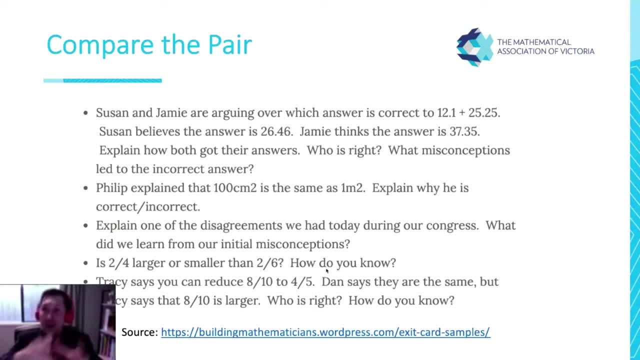 the end of the lesson or towards the end of the lesson, she got the groups to come up and share their strategy with the rest of the class, so they all saw it from different ways. i thought it was just such a great way to go through and and attempt. one of these questions was one question. 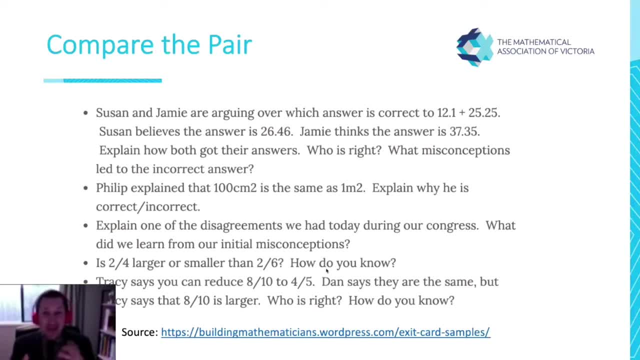 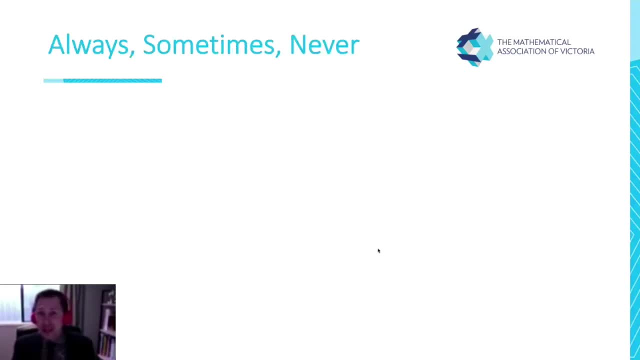 for the whole lesson. but what actually? what came from that was just such deep understanding about what was going on. another approach that we could use to answer these questions was to ask students what was going on. another approach that we could use is: um- and i have students um, that would say: 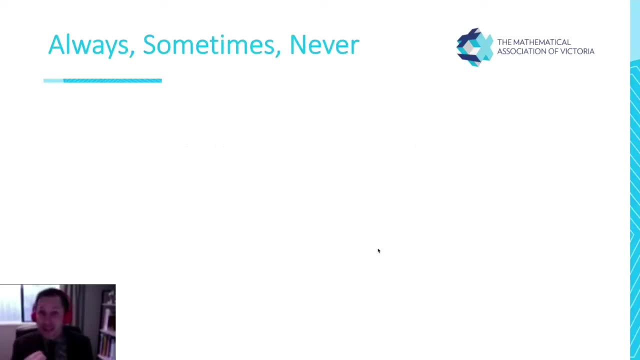 it's just the same. yeah, great, and that's the. that's the process, i guess, of trying to then bring in that reasoning as well. um, so there's like it's about going: okay, well, tell us, why can you show us? can you show us another way? um so, another strategy that we could use is always sometimes. 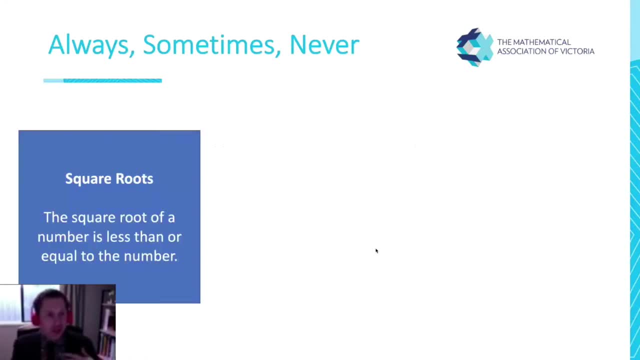 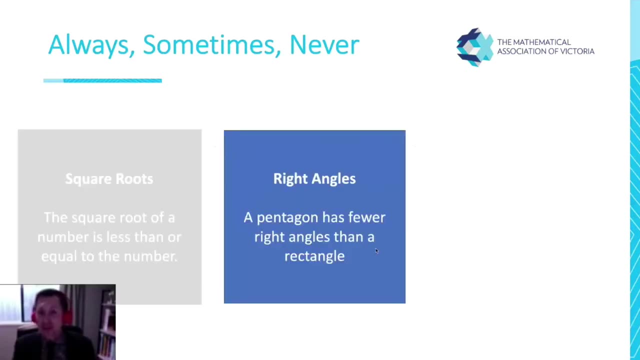 never, so i've just got a couple of these ones up. so square roots: square root of a number is less than or equal to the um to that number. right angles if you want to use the square root of a number is less than or equal to the number. right angles if you want to use the square root of a number. 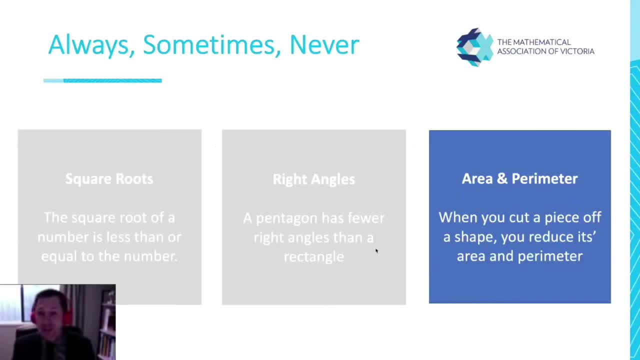 area and perimeter. when you cut a piece of a shape, you would reduce its perimeter and area. so with these questions, are they always, sometimes or never, true? i don't know about you guys, but when i came across these questions i thought, oh my gosh, i got it like everything started running. 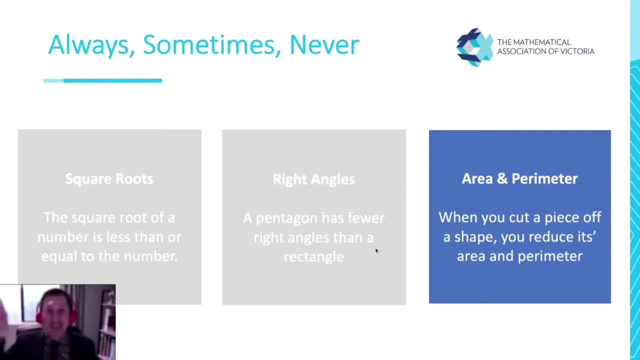 through my mind and- and yeah, i can see people going love it, wow, like there's just, it's just so powerful to start thinking about things deeper rather than just saying, um, yeah, you know a square root, it gets less, but then does it when you go less than one, it doesn't. 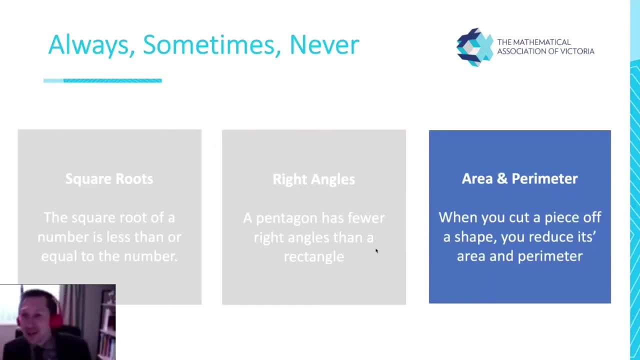 always happen so. so it's better for them to think about it before. have you always- sometimes never- for um number talks and remote learning? yeah, brilliant, awesome, enrich, yeah, they, these ones. um, enrich does have a number of them, absolutely so i'm just looking at the time. great, we're traveling. 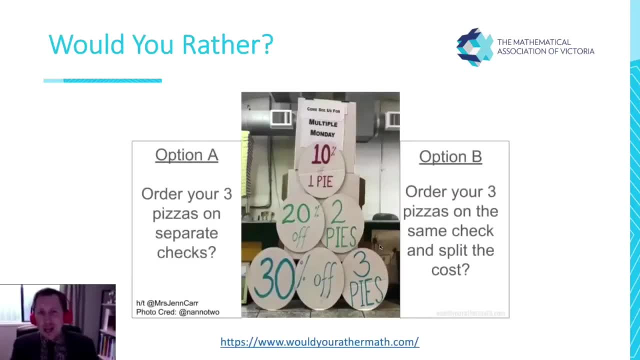 along nicely. another one that i, uh, quite like is the would you rather. now, this one comes from america, but this website- and this website is based on the word would you rather- which is a- is based in america. so it's a little bit interesting, because you got pizzas here, but then 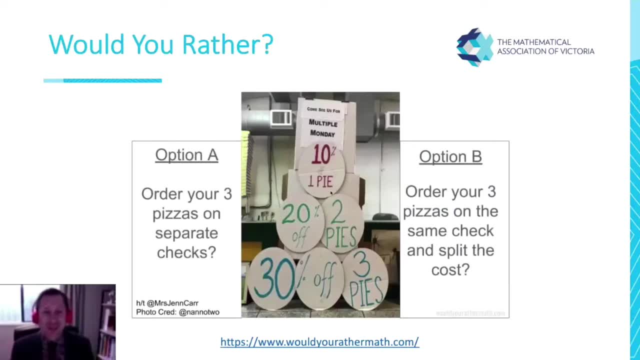 they talk about it as being pies and that might be a bit confusing for students, but imagine that you went with three friends to go get pizza and this was what was an offer. the question is: would you rather actually, um, buy the three pizzas on separate? you know bills, so would you rather just? 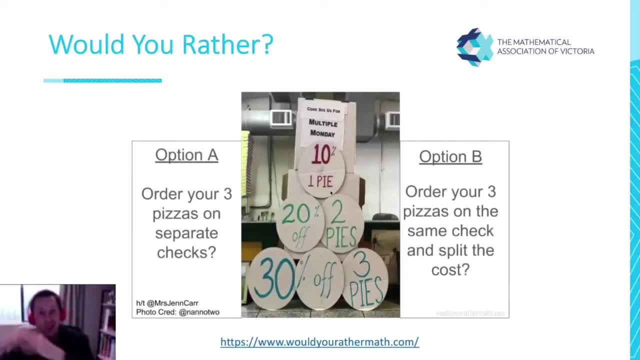 go, i'll get one. oh, you get one and you get another. or would you rather get all three pizzas on the same bill and, and um, split the bill once you've done that, like have a think about that as you go through and do that, and then how would you prove that that's the case? it's this once again. it's the reasoning. 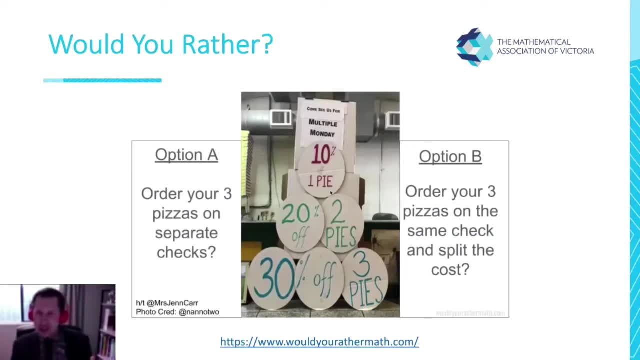 that comes through here. it's the thinking about: okay, well, i think this, but why do i think it all right? so what would we rather? would you rather option a or option b? and why- feel free to put that into the chat as well- option b, and why is that, jeremy, feel free to, because, because that's the whole, the whole point. 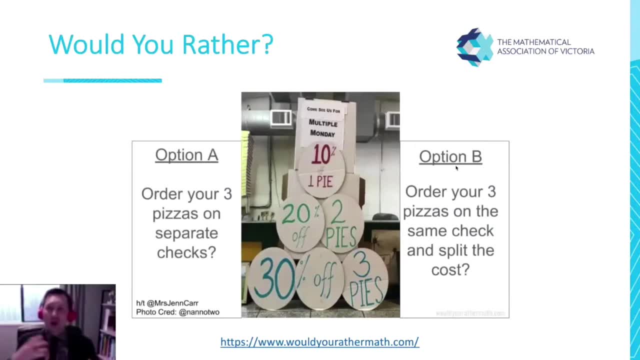 with this and i know it's quick to put down the bits. i'm actually asking for a lot in terms of chatting, but yeah, it's all about reasoning. so it's not just giving the answer, but why would you do it? b, you will receive a discount which is shared amongst all three of you. okay, cool. 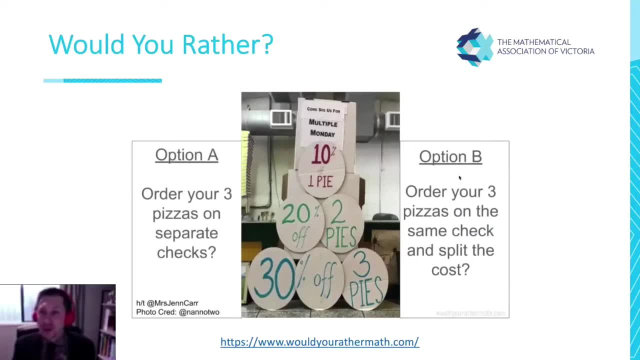 sarah, would you be able to jump on the mic and share? you're thinking a bit more about that, if that's all right. okay, yeah sure, um, if you all order your uh pizzas separately, then you'll all pay full price, but if you all order the pizzas together, then, um, you'll get your 30 off, and then, when you separate, 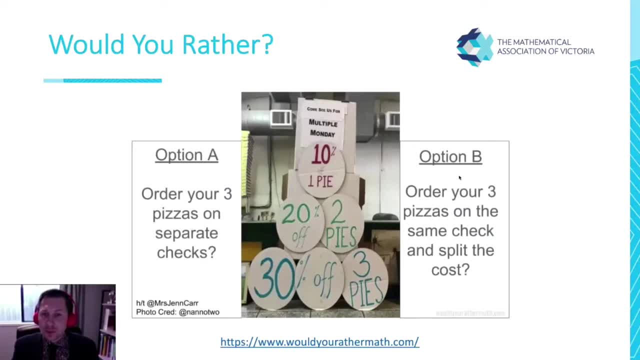 like you know, divvy up the price, then, um, you've all essentially taken part of the 30 discount. okay, can you? can you give me maybe a bit more information, maybe with some numbers or something like that? oh gosh, it's the end of the day. 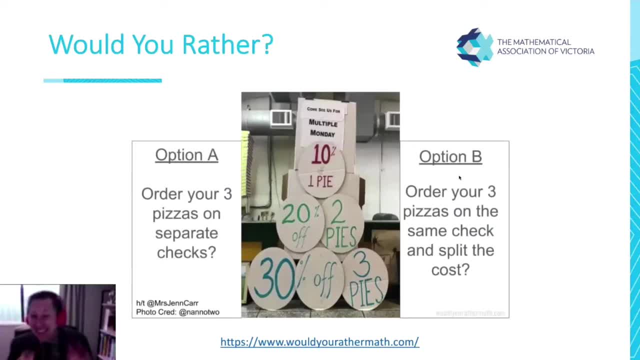 of the day, i don't use my brain that much, that's okay. i'll let you off to it right now. that's okay. is there someone else who maybe would be able to share? so, um, depends on if there's three multiple buy discount, all of them are the same price. ah, so maybe they're not all the same price. 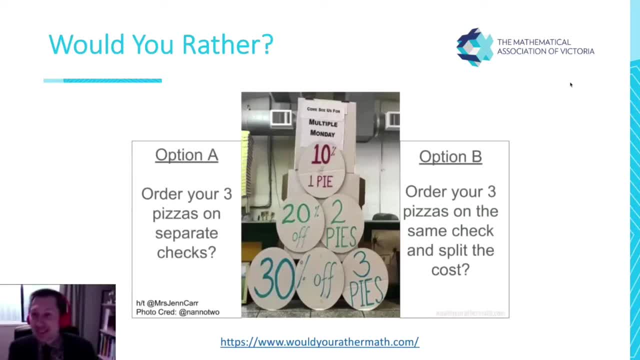 oh, yeah, so jump in. someone was just about to say something. yeah, so if you order one pie or pizza or whatever, um so if one person orders that, they get the 10 off. so if the pizzas were ten dollars, each person would pay seven dollars for their pizza. but if 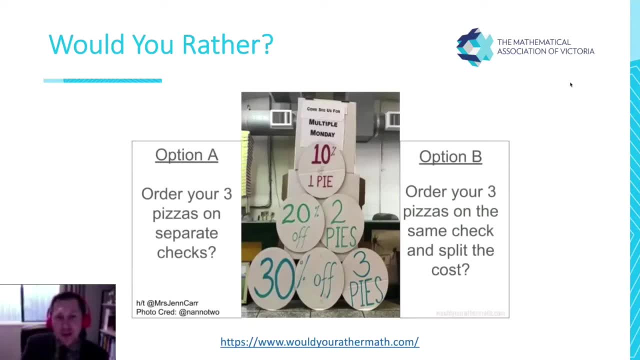 they went in and they got 20 off for two pizzas, then are they not just getting 20 off the total price, which is going to be the same discount anyway, and then i suppose then the question would be: when you divvy it up between each person, would they get then less, which is yeah, because for 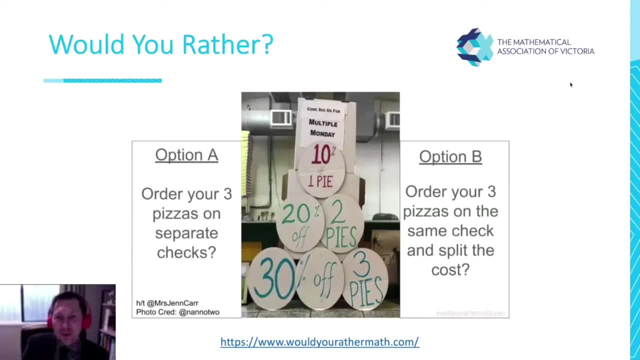 instance, if they got 30 pizzas, if they got three pizzas, which was thirty dollars, um, and then they got a discount of nine dollars, they'd have 21 to pay, but each person would still pay seven dollars. so if you're saying, you're saying that this one here down the bottom would be seven dollars per, 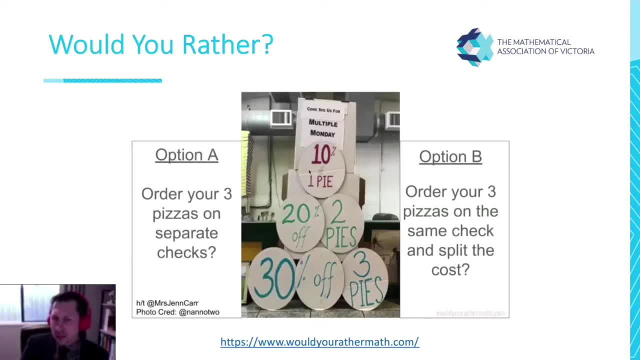 pizza, yeah, whereas, yeah, whereas- the 10 off, they had to pay nine dollars each. if the pizza was ten dollars, ah right, cool, nine dollars each, or eight dollars each, but then if they all got three, they'd pay seven dollars each. yeah, nice, absolutely, and that's, that's so true. and then, then we could start. 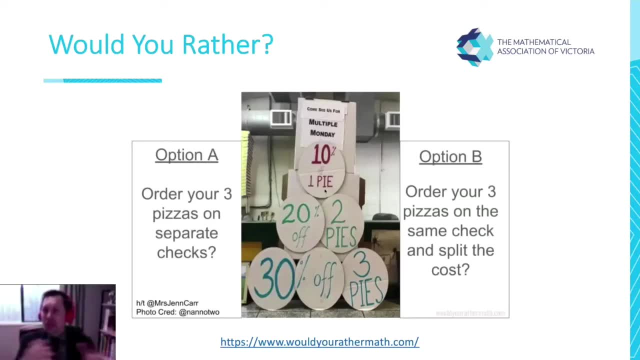 thinking about: okay, well, we've now done it in terms of ten dollars because that's a nice round number, you know, a great place for people to start. but could we then do it in terms of algebraically, like, how might we represent what's actually happening here in terms of with algebra? 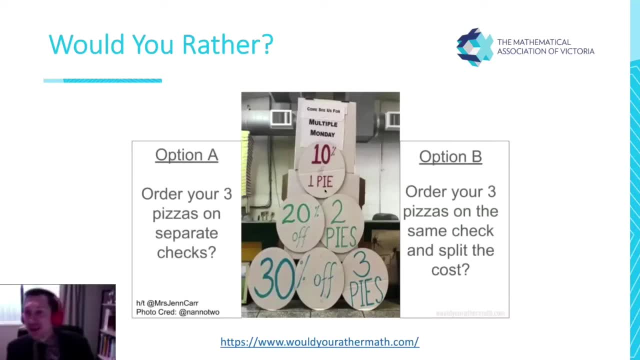 like there's a bit more going on here. i'd be more concerned about ordering pizzas from a pie shop. that's fair, simon, i probably would be too. i guess this is what the americans do, but uh. but yeah, i would be the same, right. but we'll leave it there because i want to go on with the next one. we'll. 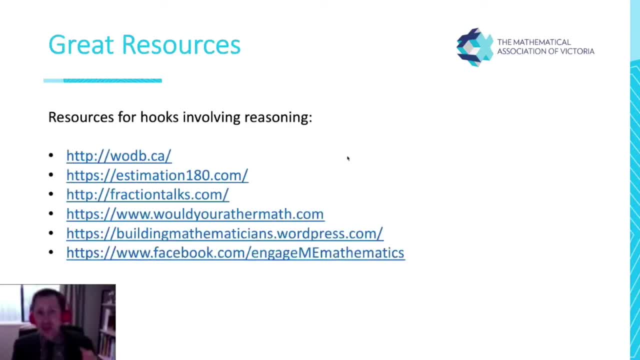 go on with the last little bit, so resources for hooks involving reasoning. so hopefully what you saw in that last little bit was us going through and and it was really addressing okay. well, we can't always do the fun rich, open-ended math lessons, because we do have to address the 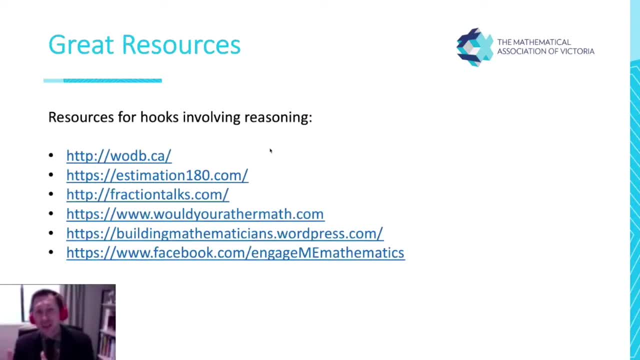 curriculum. but hopefully you saw in those strategies that we just went through- and i'll share them with you again in a second- is: these strategies help you to address the curriculum dot points but also bring in reasoning at the same time. all right, how am i going for time? 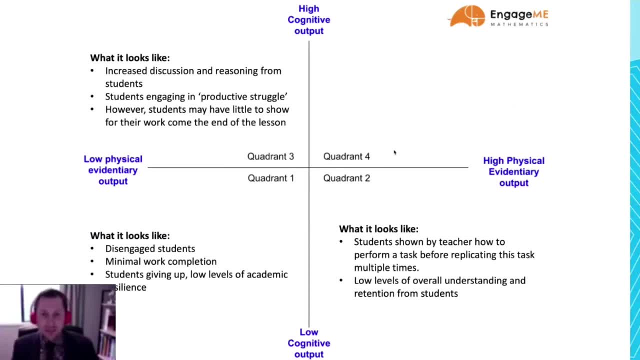 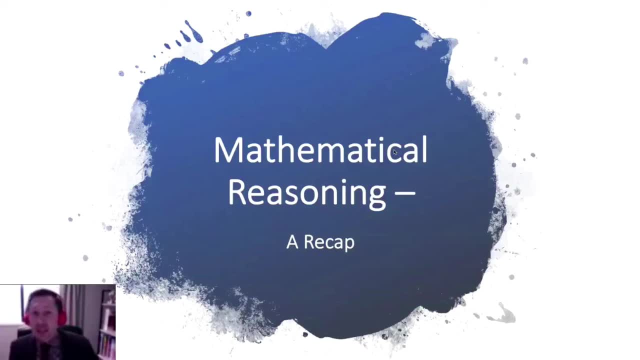 i might go skip through this bit here and i'll come back and just do a bit of a recap and then i'll leave it open for questions for the next um, five minutes, if you guys have got any, and i'll be more than happy to share my thinking things along those lines. so a little bit of a. 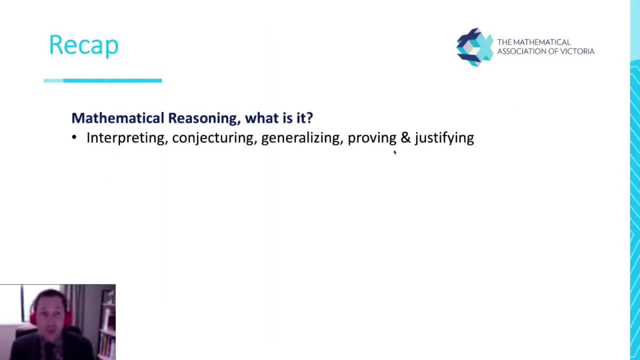 recap, at the very beginning of this workshop we went through and had a bit of a look at, well, what is mathematical reasoning? what like, what does it involve and all those things, and- and i talked about in terms of you know the verbs, of what it actually involves, but, like i said it, it really 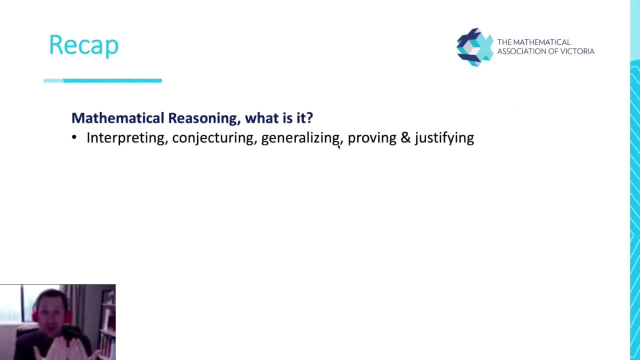 brings back to the bottom, that you don't need to have the information to understand, and then, as you're trying to make sense of the data and and what's going on, it's about taking a step back and and being able to try and make sense of that and see the broader picture, and we do that through. 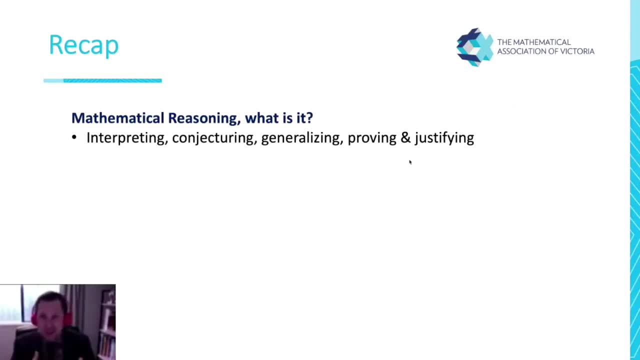 doing each one of these verbs and being able to explain it to others. it's. it's the bit, like i said before, that is, it's the meaty part of the meal. it's the stuff that that keeps coming back for more. it's the exciting part of mathematics. um, that that i don't believe the other students can do, that. 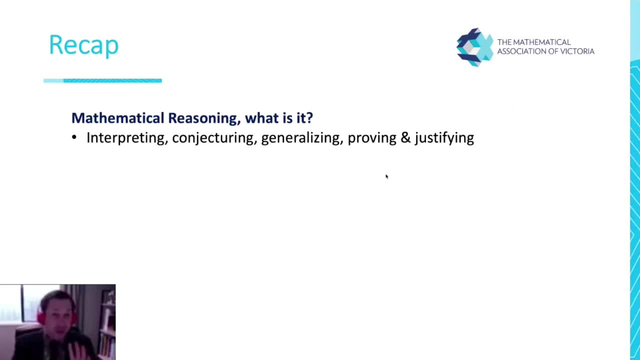 other ones necessarily involve just as much, but maybe that's just my preference. I can't comment on that for everyone. these are some of the strategies you can use to incorporate mathematical reasoning within our actual lessons. so number talks, mathematical exploration, so like rich tasks and things like that, and then the what's happening here. compare the pair always, sometimes never would. 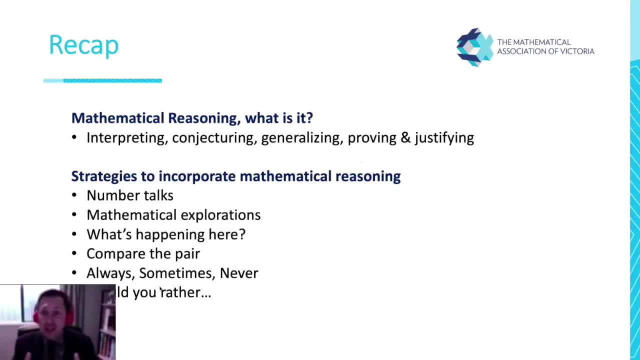 you. rather, those are the ones that I use to go through and actually explore, to go through and explore, you know, with specific content descriptors. awesome, Alex box, I've number talks. I changed my life. that is one hell of a of a pump up for number talks. it is awesome, it's so good, okay, so yes. 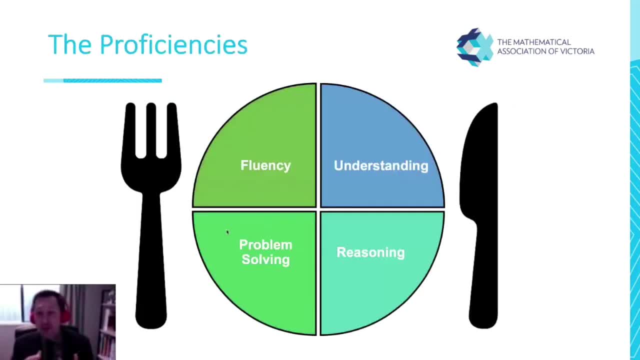 reasoning is. it's an important part, though, of the curriculum and what we do, but we need to make sure, like I said, that we address the entire plate, the entire nutritional meal that is, maths education, because if we focus on just reasoning, it can turn students off as well. so 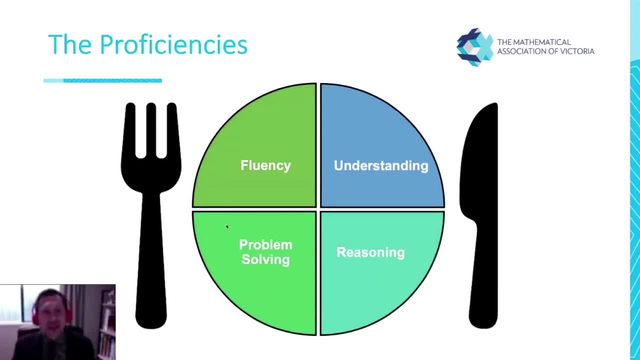 really making sure that when we look at the tasks that we teach, think about them and reflect on them and think, well, what am I actually addressing in here and am I focusing too much on on understanding or fluency or problem solving or even reasoning, and do I need to make sure I'm addressing other? 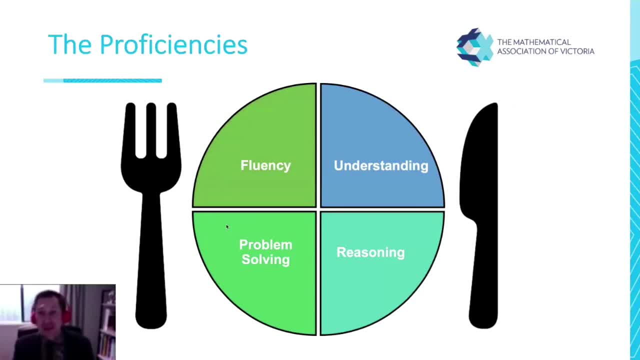 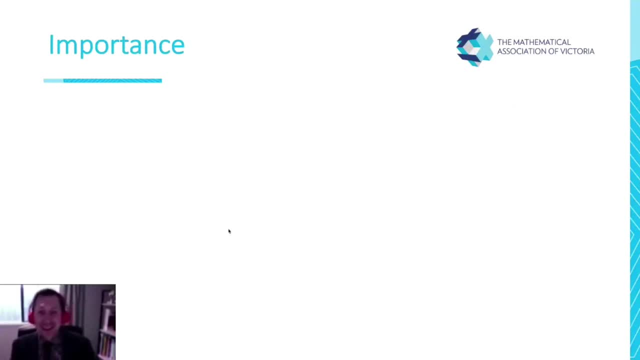 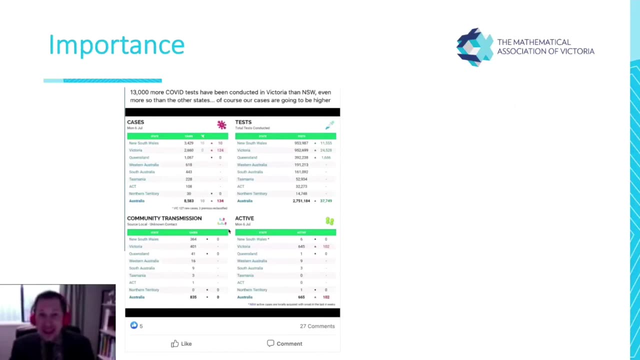 parts of of the meal that we need to do in terms of the proficiencies now. why is it important? I'll finish on this. so a couple of months ago, I came across a post that that was from a fellow maths legend, and she put this up and and she shared this, this stat, along with some of the data here. so 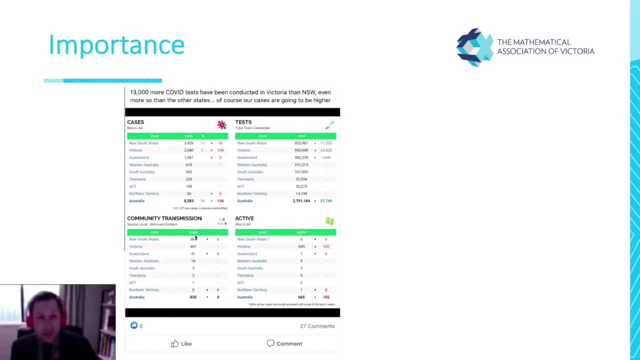 I'm going to give you a moment to go through and and have a look at what you can see here, try and make sense of it- there's a lot there to take on- and then have a look at what one of the replies was from- from someone as well. so I'll give you a oh yeah and which one doesn't belong? great one a. 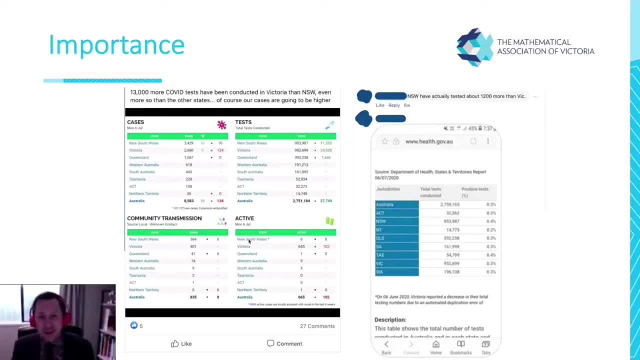 couple of. I didn't remember to put that one on. have a look there, though, and try and make sense of what's actually going on in this post on Facebook. okay, it might be. yeah, all right, fair enough, it might be a little bit too hard for people to read. 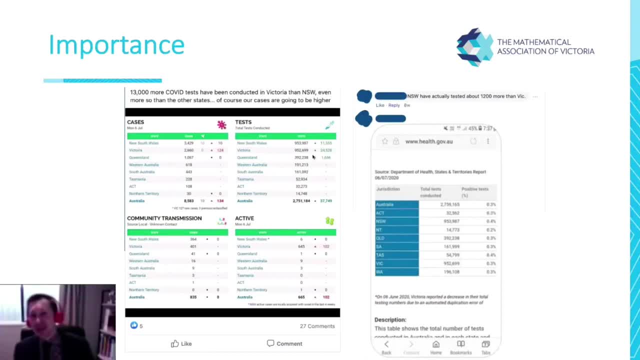 that's fair, okay. so I'll just quickly summarize. what was happening is: essentially there are there are two, okay, cool. so Sarah said the first post was talking about daily tests, not overall tests, and the impact on an increase in rising cases. so essentially, what's what's sort of happening is? 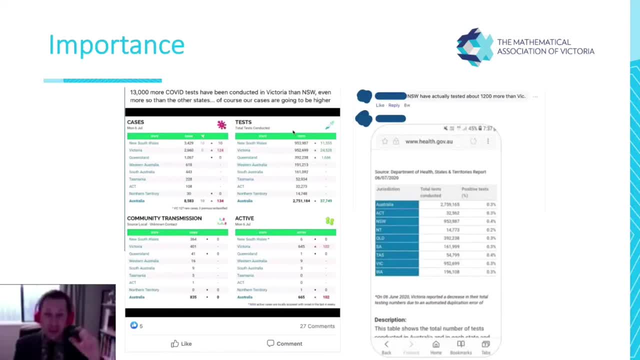 there was a post that was on Facebook, um, and- and the person who posted it talked about: okay, well, we had more tests done in Victoria than in New South Wales. so because there was more tests done, we were more likely to pick up on on people who actually had coronavirus, because obviously we're doing more tests. but then the 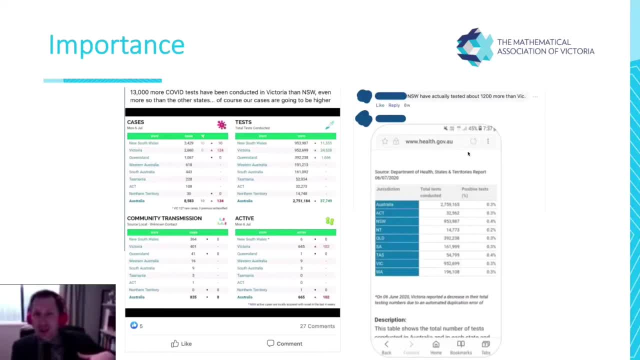 other person came through and said: no, no, there hasn't been more tests done in Victoria, there's been more tests done in New South Wales. now, in fact, both were correct, but they were both arguing different things and and um. when the person who originally posted it went through and did this, they um and the other person. 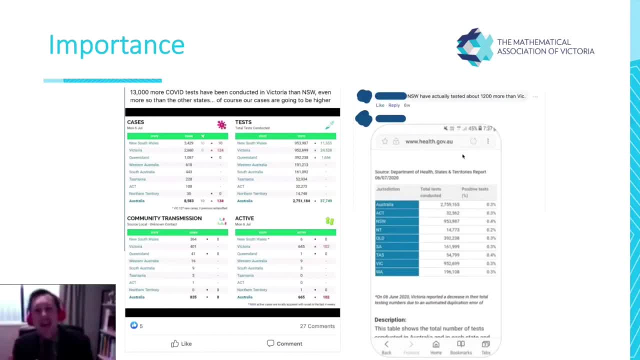 kept coming back. they explained their thinking, but the other person was so stuck on their data because they didn't. I would argue that I didn't quite get what was happening in the first piece of information. now, why is this important? well, especially right now, when we're looking at people. 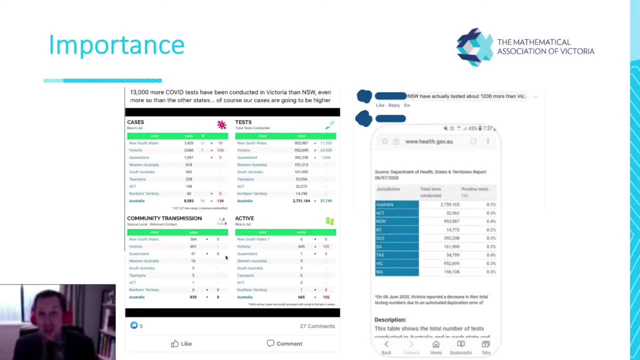 who need, like you know, people need to be able to read and interpret and make sense of a whole lot of facts and figures that have been thrown at them. and and if we don't teach people to be able to reason and to be able to look through things and see, like I said, the 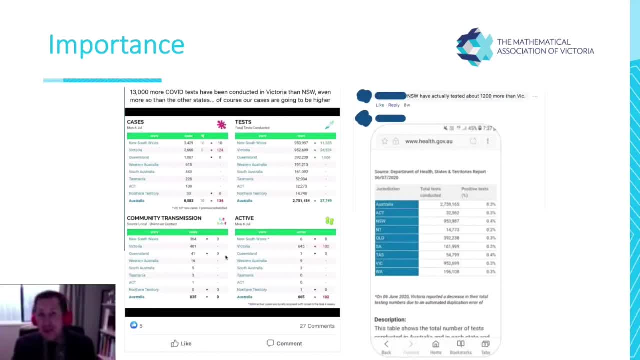 forest through the trees, then then we do have that. we run that risk of people not really making sense of what's going on. and you're right, and some people like it says we need to define the population. so so they could, we could have certainly gone through and maybe defined some things a bit better in the 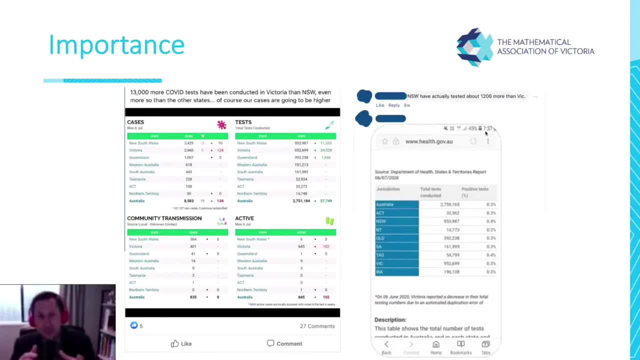 first instance, but then they did do that later on in the post. but it really is a matter of okay explaining the reasoning and really understanding what's going on. if we can't teach or if our students can't reason, then we run the risk of having these issues that people don't understand. 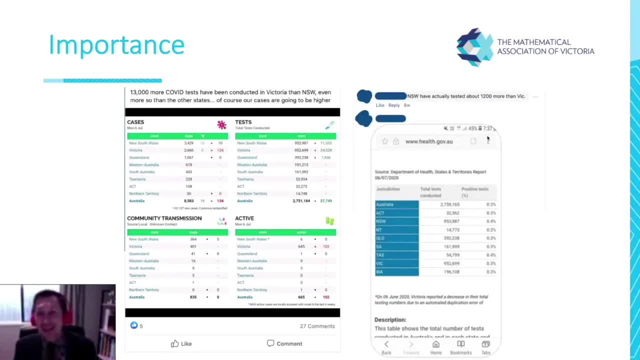 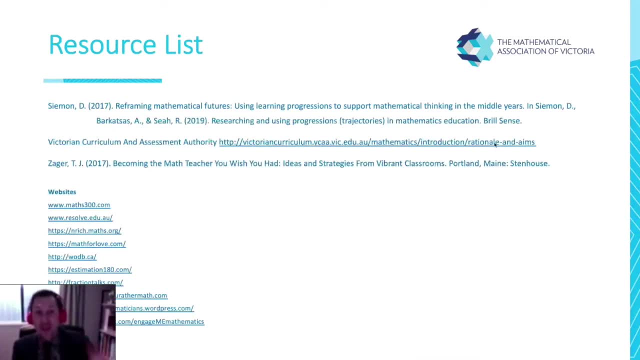 what's actually been put in front of them and we and we know, now more than ever, that that's really really important. so here are some final resources, that and this is everything that I've gone through today. it's all on the one slide so you can go there at the end and and do that, and also I would 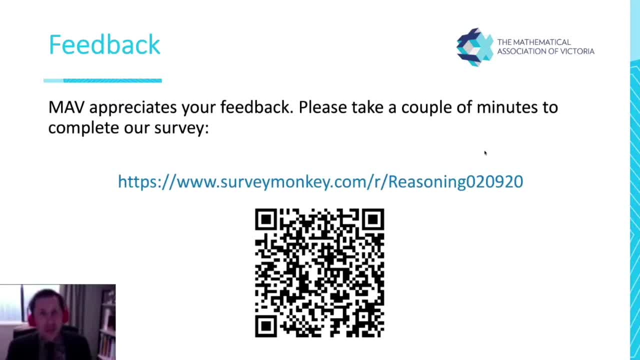 really love your feedback on what you thought of today. please feel free to give me constructive criticism, like anything that I can improve on, because I'm really passionate about getting better in what I do, so I would really love any kind of feedback along those lines. but other than that, thank you very much. if you've got questions, feel. 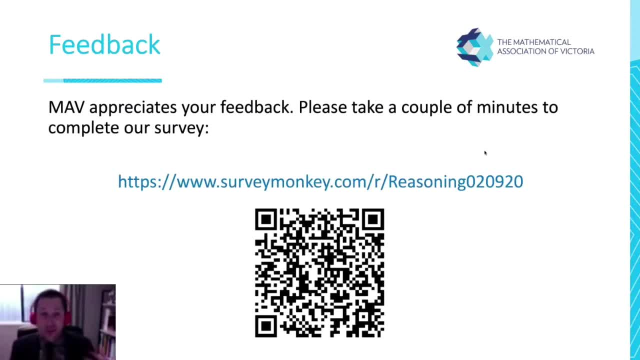 free to put them into the chat. I'm more than happy to to go through and answer these for the last few minutes or a last couple of minutes, but also, yeah, like I said, thank you so much for your time today because I know that, like I said, you're busy people and to for you to spend an 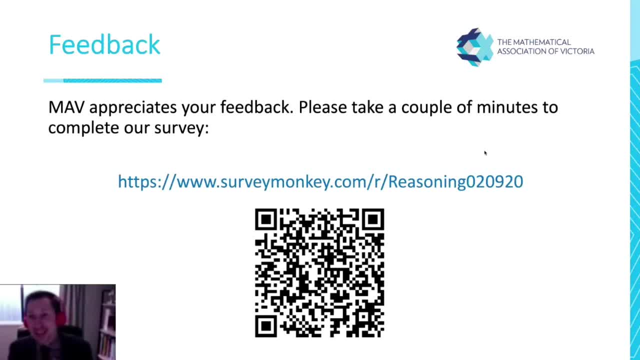 hour here listening to me. it really is a pleasure to be, to be with you guys today. thank you, um. uh, the green textbook in the Miland was. I'll put a link to it. let me, um, find it. I'm gonna. oh, actually, let me. it's this one teaching mathematics foundations to middle years. that's the, uh, the. 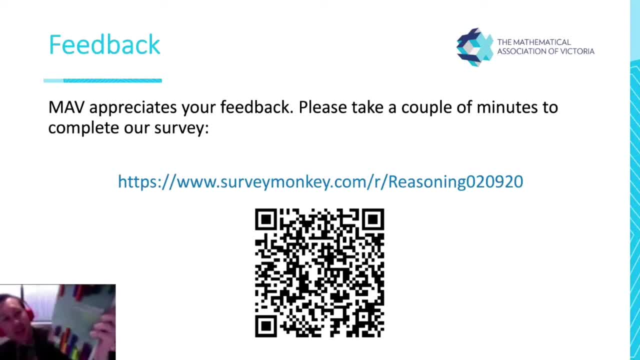 green textbook. so what was it called? sorry, Tom. uh, it was teaching mathematics. yeah, foundations to middle years- awesome, thank you. no worries, now the chat's moving very quick, so if you've got other questions, feel free to um to chuck them in again and I'll go through and answer them if I miss it. 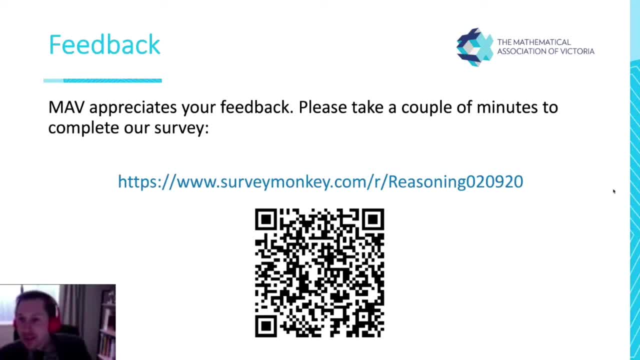 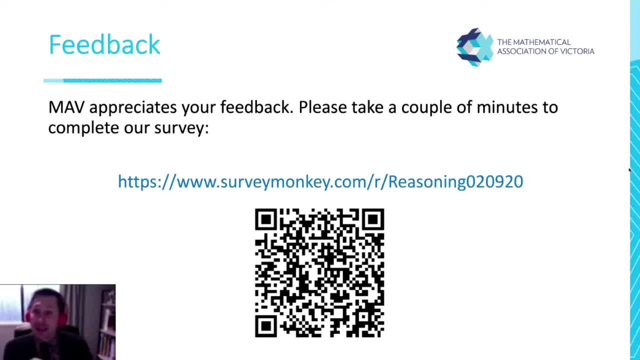 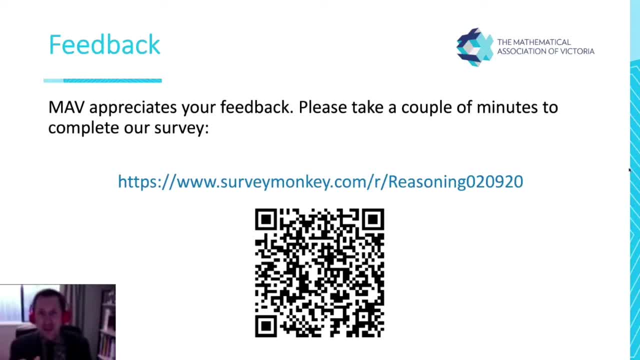 skill that you're developing or you're getting them to do, as well as the reasoning. and and if the reasoning is just getting them to the point where they're understanding that skill, then I would say no, they're working. they're actually working at that standard. so you've got to think. 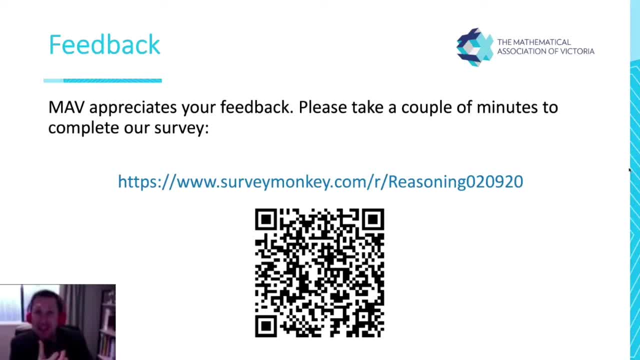 they doing with the skill? are they taking it further or are they just getting up to understanding that skill? how is the reasoning being used? hopefully that answers your question, okay. uh, Savita, in terms of the Facebook animations, yes, so very exciting stuff, you um at the moment, 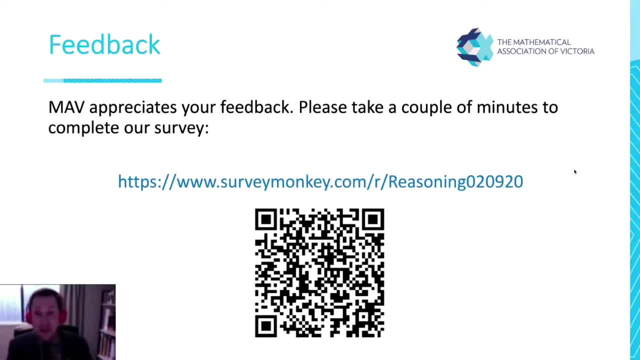 there is an opportunity for you can. you can go through and subscribe to my mailing list. if you look at any of the animations on um the Facebook page, if I subscribe, you'll find that there's a link to subscribe to my mailing list. you can do that. at the moment, though, the exciting part is 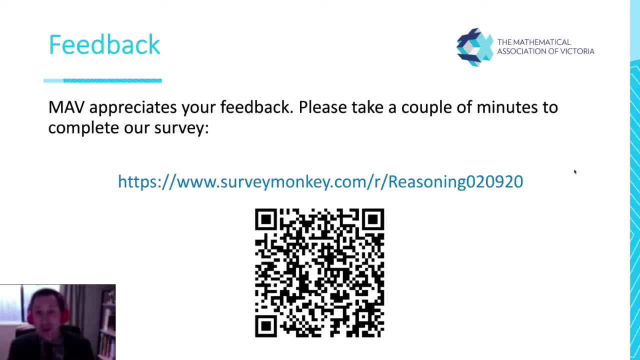 we're actually in the process of putting together a website that people can subscribe to um in, and hopefully that'll be ready in the next month or two. it's we're on the process. we're in the process. now we've got someone and hopefully we'll get that up and running really soon. so they're not. 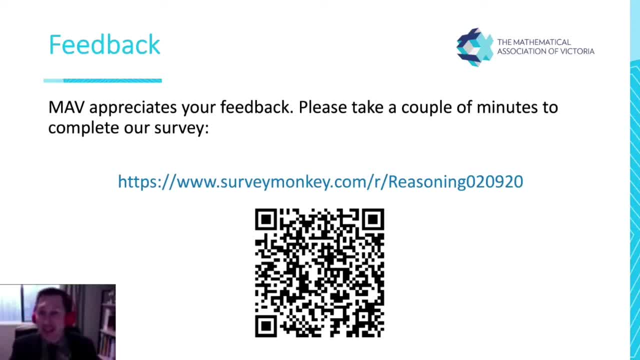 in a place where everyone can get to them all at once just yet, but we will get to that point soon, so I'm sorry for it taking a little bit longer than what I would have liked. uh, yeah, so the engagement maths animations at the moment are only on Facebook, but you can still subscribe to our 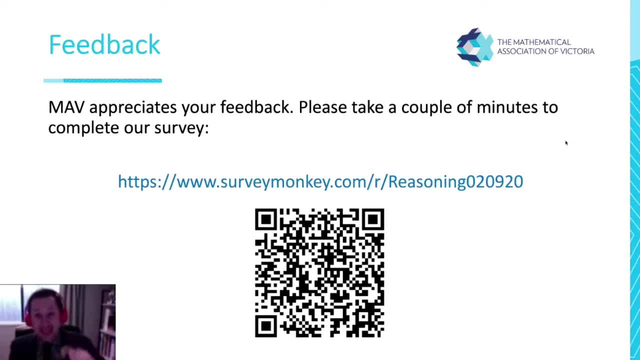 mailing list for free. um, and I send out our latest animations each week, the, the latest, the. we will have a website up and running in the next, like I said, month or two. um, where will the slides be available? at the end of this? they'll be emailed through to you. uh, do you do much with Craig Barton? I'm. 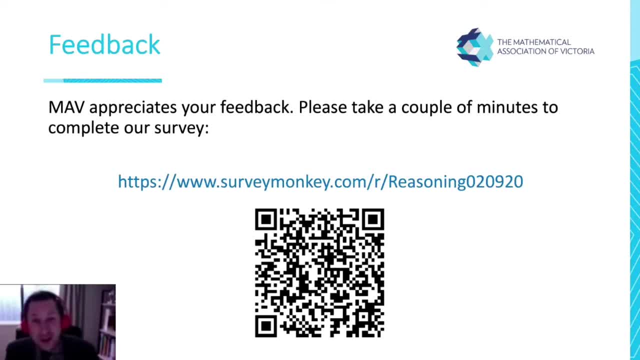 reading his book now. I wish I'd taught Matt. you know what I've heard about Craig Barton. I haven't looked at too much of his stuff, but it's on my list of things to do. do you think we can address all of the curriculum if we focus on the proficiencies? Emma, great. 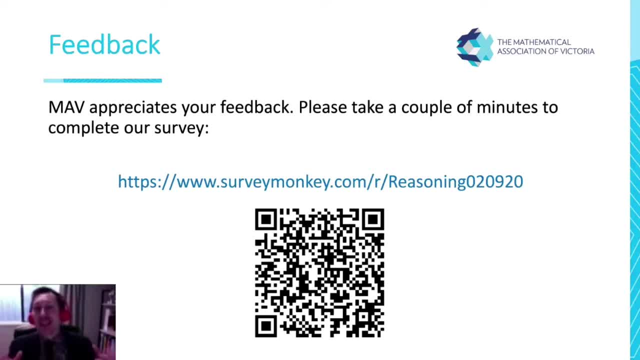 question, really great question, and yes, I do, but we've got to be clever in terms of how we go through and do it. so I would start off by doing a bit of an audit, or just keeping track, roughly if, by looking at the curriculum and saying, okay, well, what am like, what is this activity that I've 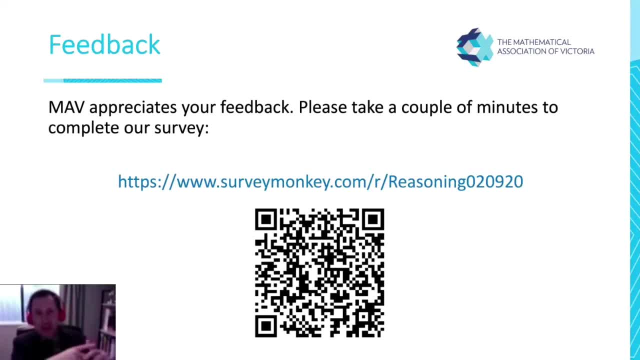 just done here. what is that actually doing? what am I addressing? am I addressing um fluency? am I addressing understanding, like what are the main things that I'm doing, and maybe only choose the two to address? most often students will address all in some capacity but think: well, what is the one that? 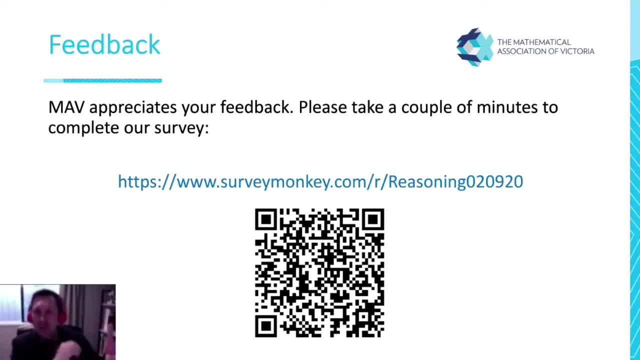 how am I like in the way that I'm addressing this activity now, what is it most addressing? and then do that for a few activities over the space of a couple of weeks and just keep an audit of what's going on and you'll get a very quick idea of what you're spending most of your time on. 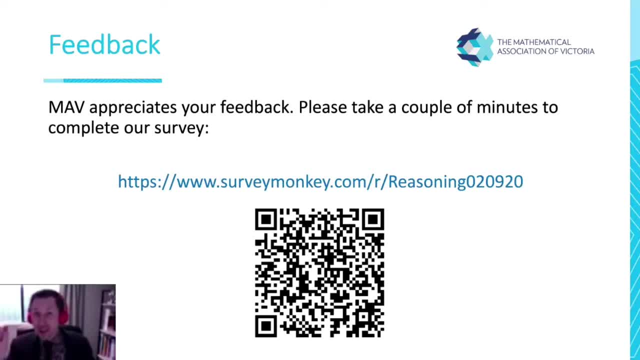 I really believe that it is possible. you can ask a question, one question, and change the um, change the proficient proficiency that you're addressing by changing the way in which you ask that question. and maybe that's a PD for me to do another time, but it's absolutely possible. where do you access?